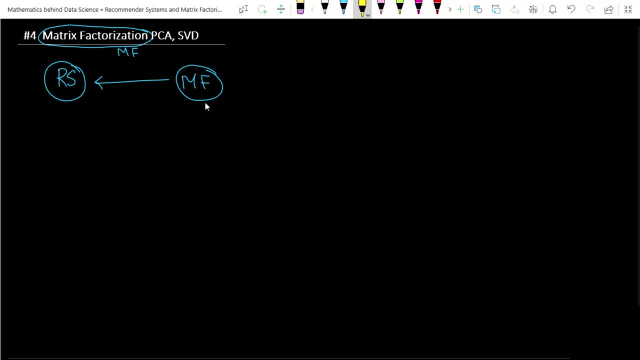 video. we will trying to first thing that in the other main main agenda of this video is: first we have to learn what is. we will learn what is AMA, what is matrix factorization. So we will learn first it. and and second agenda is we will connect with this, we will connect this matrix factorization technique. 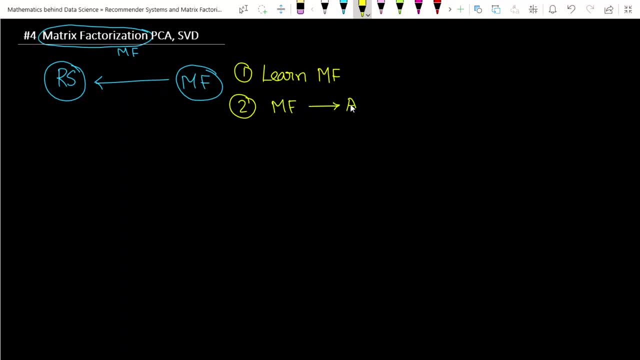 to the PCA and singular values decomposition technique. We will connect it. The matrix factorization that we are going to learn. it is a it's a technique in applied mathematics chapter. So let's start. it's a technique in applied applied mathematics. it's a technique in applied mathematics. 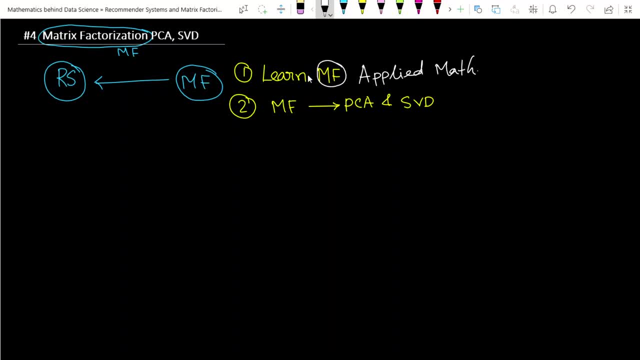 So let's start. so first what each position is. what is matrix factorization? let's try to understand what is matrix factorization. what is it so? the answer, in fact, that arises here. so let's try to understand through this example. suppose a is a matrix, a any matrix- supposedly it's a any matrix. 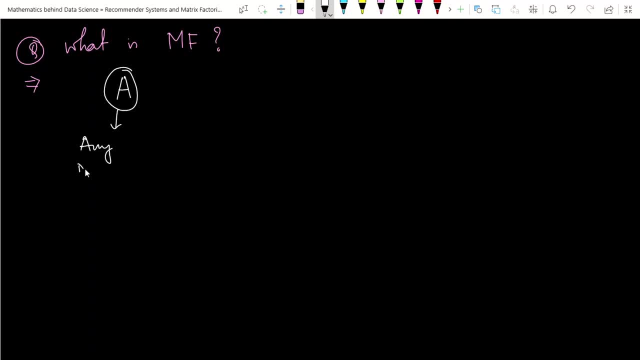 suppose let it's any metric. now, first job that we have to do: we have to convert this matrix to the multiplications of as some other matrix onwards. suppose let's check c, b, c, d. we have to convert. so these are means, these are means. the job is the we have to convert. 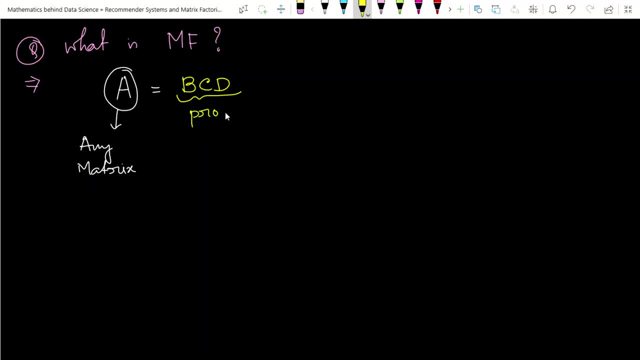 this matrix a the product of other matrix. product of other matrices. we have to chop this, doing this job, so that the the product of other matrices that we are going to discuss, that they have another name: the matrix decomposition means we have to decompose this matrix. so we have to decompose this matrix, we have to. 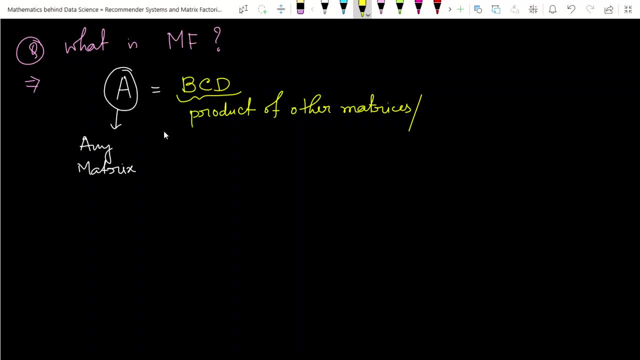 convert this matrix into the other matrix. so because of this reason, we call this technique as a matrix decomposition. okay, decomm, matrix decomposition, okay, and if you take, if you take, ah, matrix decomposition, so you have to take b into c for that in order to get this matrix decomposition of the matrix. 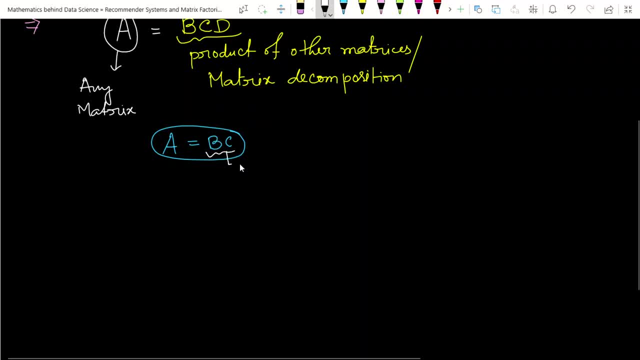 now let us take a look at, uh, another example. supposedly h equals 2. i have to take this example: b into c, the b, c that are called here the multiplicative decompositions of the b and c, that these things are called the multiplicative multiplicative decomposition. 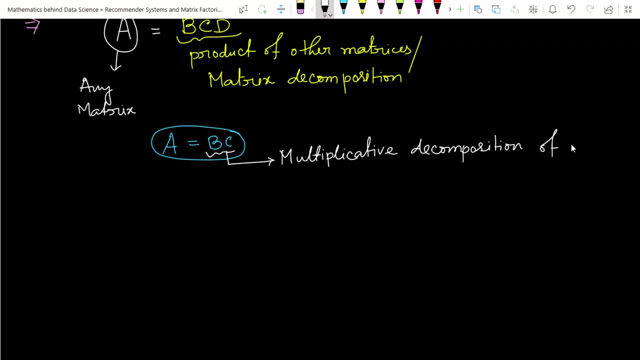 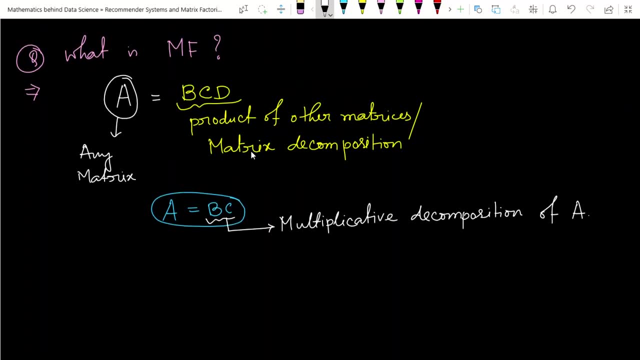 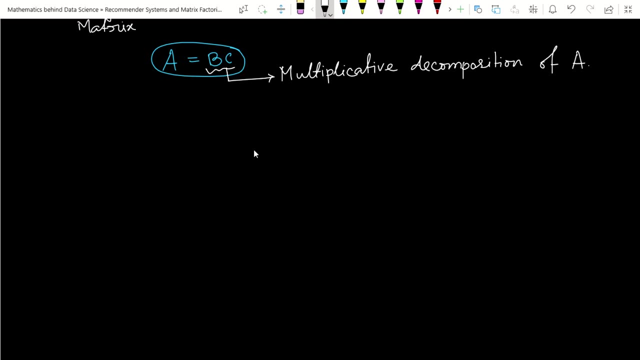 of A. that's the thing. because of this thing- okay, this technique, another language. because of this reason, this technique are called the matrix decomposition technique. I think you got the idea. now let's try to why we call this is a A matrix factorization aim it, why we call 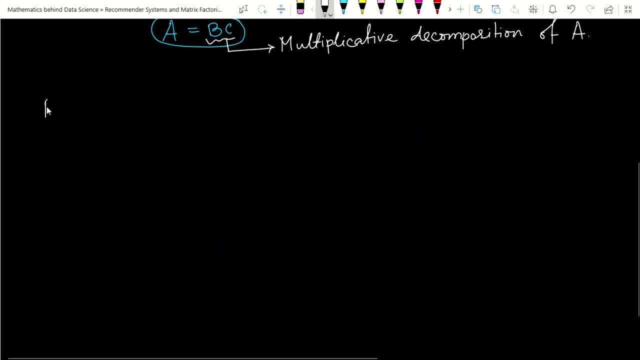 matrix factorization. why? why it is matrix factorization. now let's try to got the answer. it's right word. so because, suppose let's take. if we take is scalar quantities up, a let's take. I am taking here as scalar quantity 10.. So 10 can be written as in this form: 5 into 2 means what? 5 and 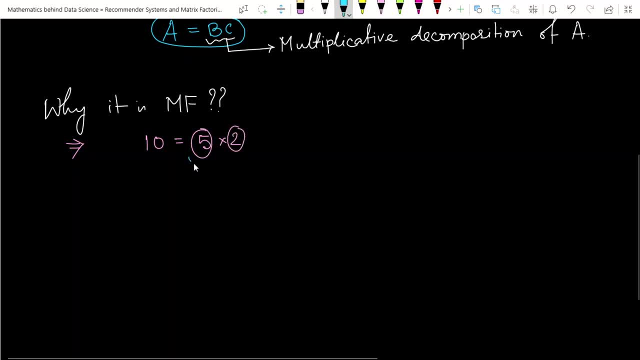 2 that we got. these two things are called the factors of 10.. These are the factors of 10.. So same reasons also applicable here. if we, instead of using the scalar quantity- if we take a is equals to b, cross c these symbols is for scalar multiplication. this: 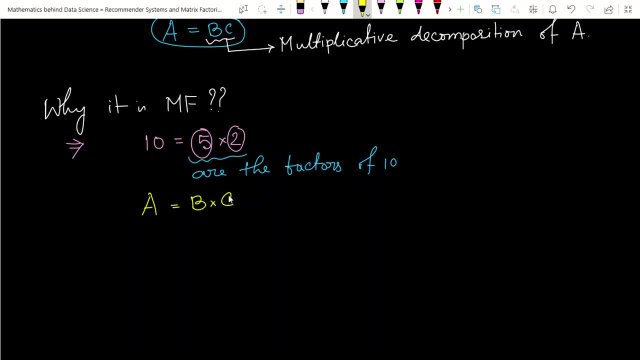 symbol is for matrix multiplication. because of these reasons, here b and c are the factors of a, Factors means the scalar factors, scalar factors, here the matrix factors, matrix factors of a. because of this reason this technique is called the matrix factorization technique. I think you will understand why we call this technique as a. 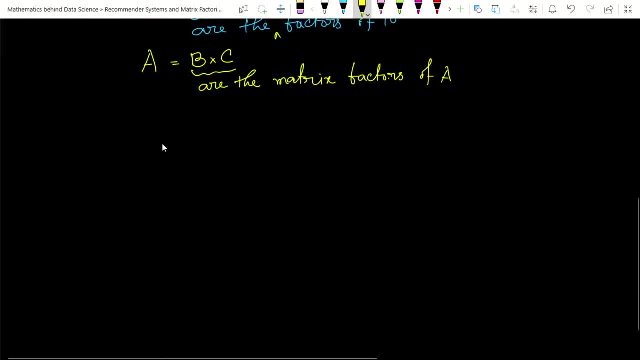 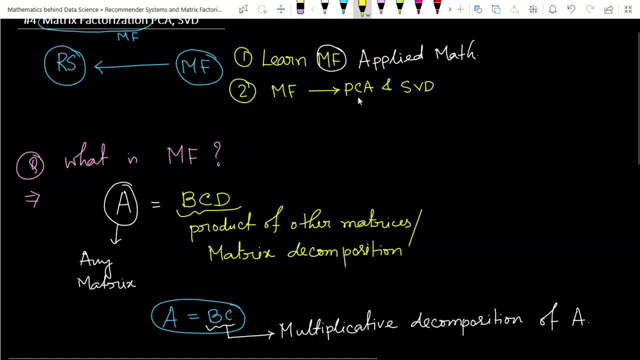 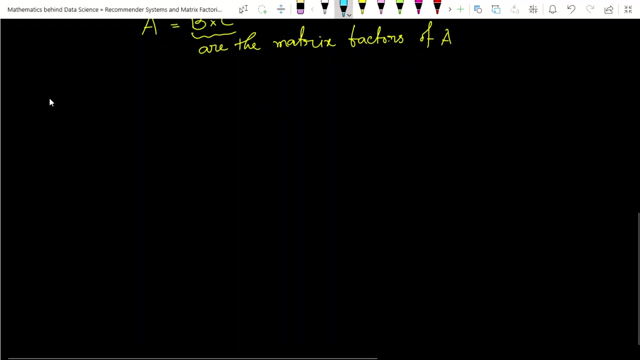 matrix factorization. I think you got the answer. Now let us try to understand this. matrix factorization technique, with the help of PCA and SBD, means principal component analysis and support vector. this is a singular value decomposition technique. Okay, let us the job that we are going to do. we have to do some of these matrix factorization. 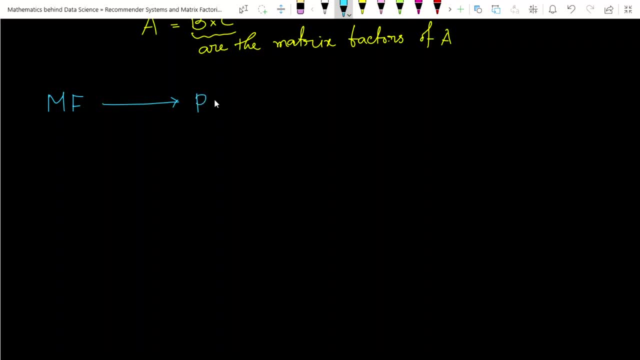 technique. We have a apply this technique to the PCA, to the PCA means: principal component analysis, principal principal component analysis and, and we will try to extend this concept into the SBD means, SBD to these things are the singular value decomposition technique, singular value decomposition. we will extend this concept. 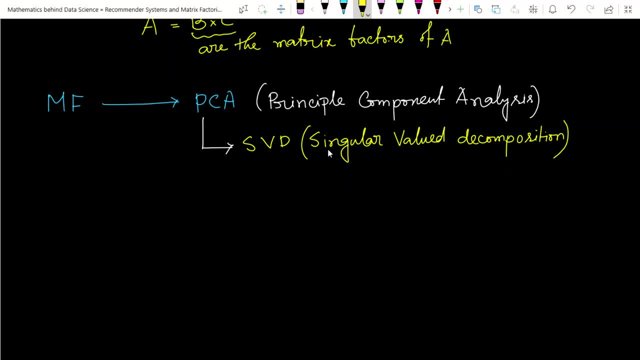 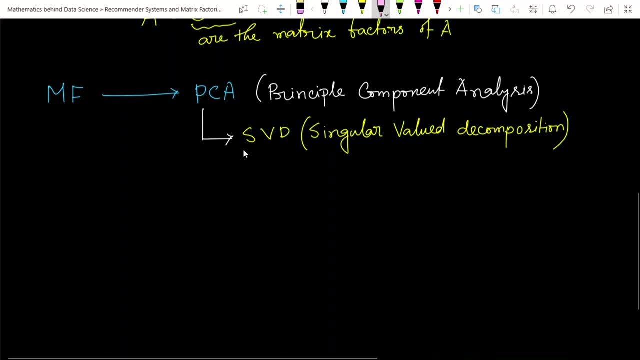 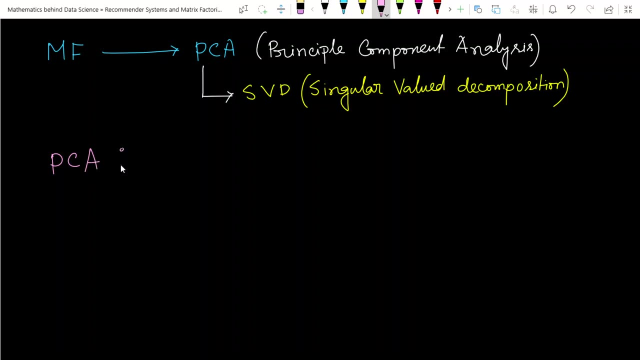 into it. okay, so let's see how we'll convert. so the first: what is the just recap? the principal component analysis first. then we will try this, try to connect this dot between them to say so. so what is this principal component analysis? what is it? what is this principal? 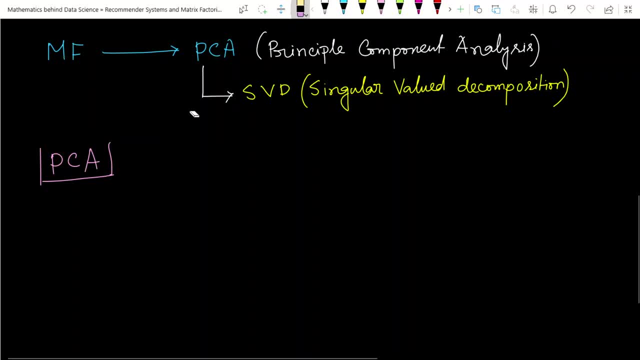 component. let's try to connect. what is it? the principal component analysis, that job that we are going to, because to convert a higher dimensional data into a lower dimension, that is the job that we have to do. we have used this principal component analysis example for for a high dimension to convert to high. 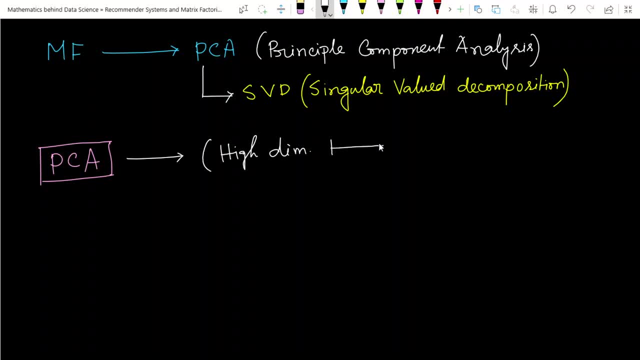 dimensional data to a lower dimension, to a lower dimensional. okay, we will convert this job into this dimension to high to low. that is the main job in pci. okay, suppose let let x is a data matrix we have. suppose let's. it has a number of data and 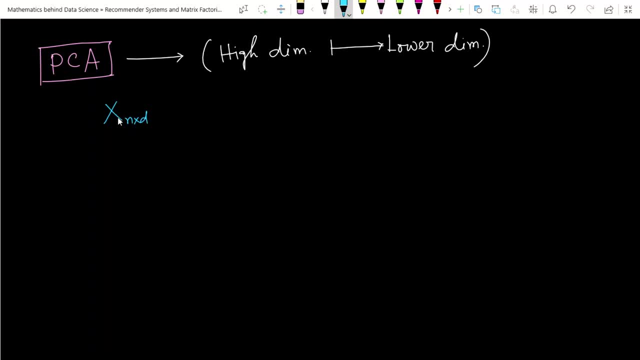 d, number of features. so, because of that, this is a data matrix. suppose that this is a data matrix. this is a data matrix and in this data we have the n is equals to number of data points, number of data points. and here d, here d. this d is equals to number of features in this data. 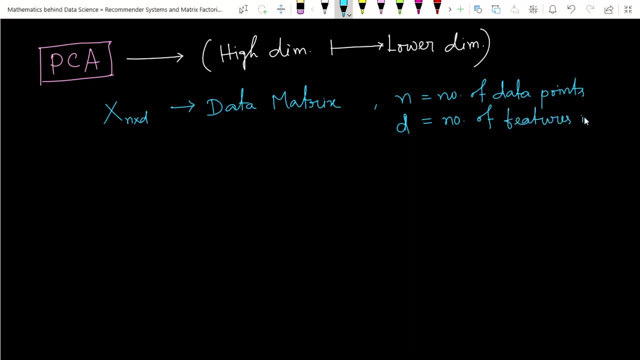 so this data matrix is a respect to the number of data points in this chain that we have seen earlier in our chart. so this is a row of elements that are consciousness, also called and theseisson inaletts. so this is the number of features and number of features in this, in this data. 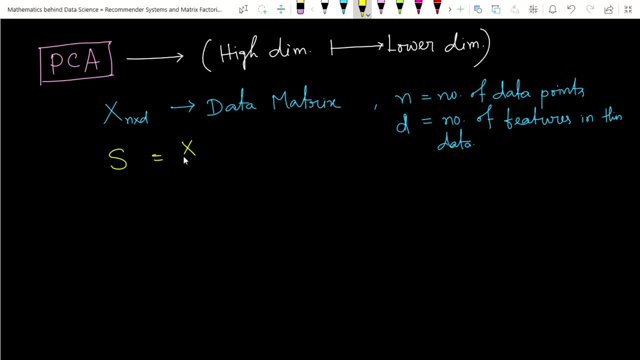 this is the sample method data matrix. now we have seen that of this transposition into x, by divided by n minus 1, these are the covariance, this is the covariance matrix, and the dimension of this covariance matrix is d cross d. okay, why these things d cross d? this is the simple covariance matrix and and we have already seen, just if you, 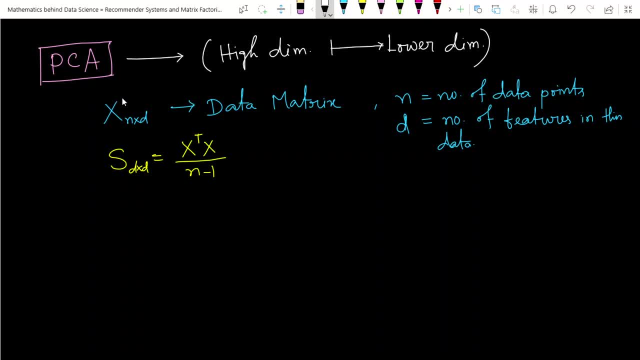 forget, just recap this principal component analysis, then you will got the answer. okay, this is the simple: the covariance matrix. this is the covariance matrix. okay, these are the why this thing? because the dimension, the dimension of the x transpose x, the dimension here is the x transpose x. dimension is n cross d. 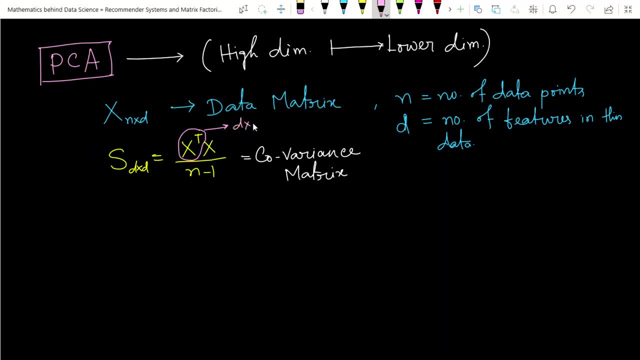 so the transpositions dimension it will be d cross, n and the x dimensional it is n positive. because of the this reasons, this is the d crossing and this, a minus 1, is a scalar quantity example. it is a scalar quantity. it is a scalar quantity, okay. this is called the covariance matrix. 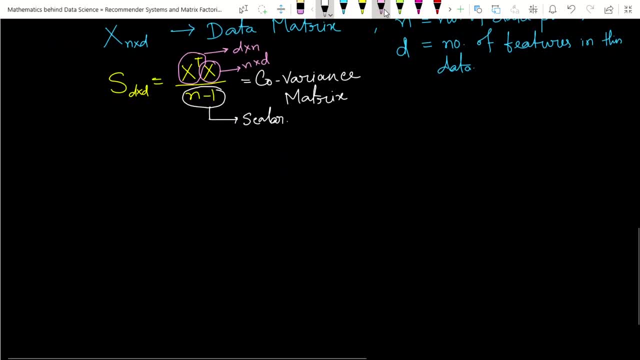 now the characteristics of this covariance matrix is: is like that, the characteristics of this covariance matrix is like this kind of characteristic we have got. so the eigenvalues of this, of this covariance matrix, matrix is: let let the eigenvalues of this covariance matrix is lambda: 1. 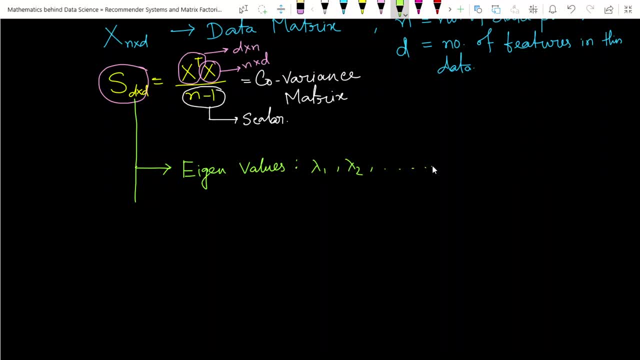 lambda 2, suppose it's the d dimensional matrix, so it's eigenvalue up to d, lambda d. okay, and the eigenvectors corresponding to each eigenvalue. let's w w, i, the eigenvector. this eigenvalues引 vector for each eigenvalue is w 1, it's w 2, it's w d. okay, let. these are the eigen values and corresponding. these are: 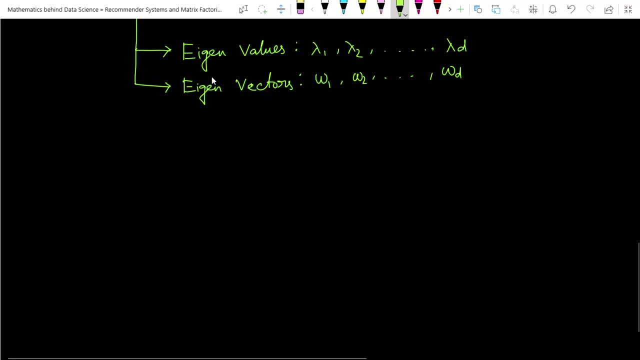 the eigenvectors for each eigenvalue. okay, right, these things we have seen. now, what is the relations between? to convert this high dimensional to a lower dimensional, that job that we have to do is to transform them, as else, from C to L, which is l, werdemenstr, in shoe numbers, which would be a actually. so this is a place where the top of the foot of the foot does not comma, as well as the� force on top of the help of the upper head of theDirector, right. so this is the vanishing effect, this value in the v value of this match point, the whisk vector as well as which, again, is it tota? it�, it is in your equation, but a little bitizada. 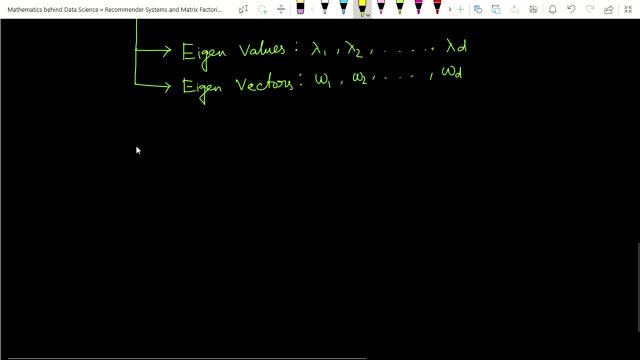 to a lower dimension, that job that we have doing, that we have to do. suppose it's the d dimension. now we have to convert this into a d dashed dimension. that is the job we have to do here. and d dust must be the lower value than t. e just must be a lower value then. so how we'll convert. 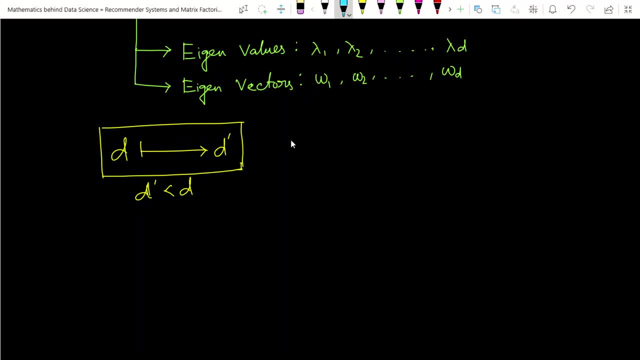 we have to top d dust lambda size. we have to choose. we have to choose top means according to the increasing order: top d dash lambda is to stop d dash lambda is. we have to choose it okay and corresponding its w is corresponding its w is will be its. 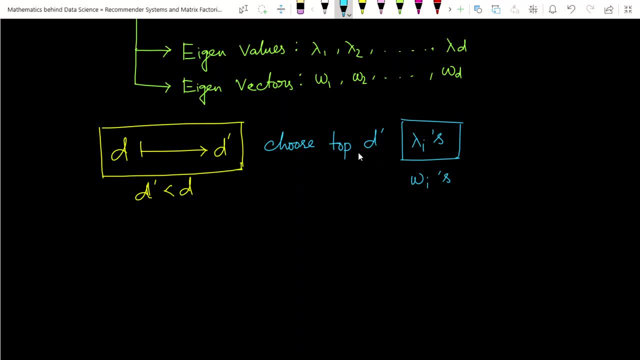 wis will be its eigenvector. okay, eigenvectors. okay, according to this eigenvalue: tops d dashed eigenvalue. we have to choose the eigenvalue. very simple: using this technique, we have convert this higher dimension to a lower dimension, so just we have to find the eigenvalues and i can make that's. 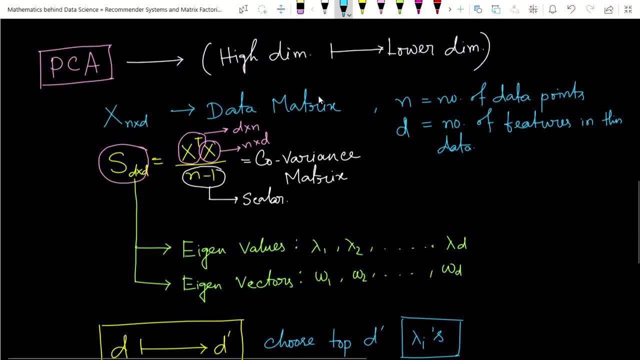 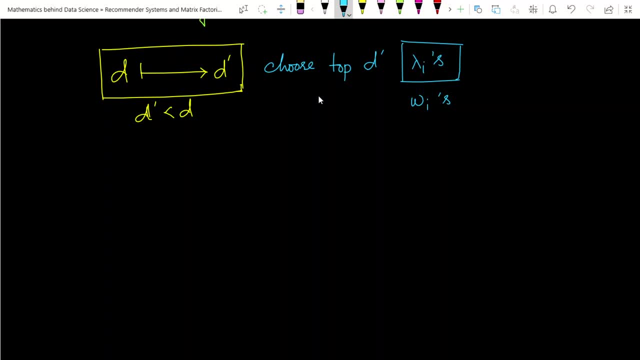 the job that we have to do. okay, that we have seen in pca. okay, this is a simple principle: component analysis. that we have seen. now let's try to connect this principal component analysis technique to the matrix factorization how we'll connect with this thing. okay, let's see step by step. 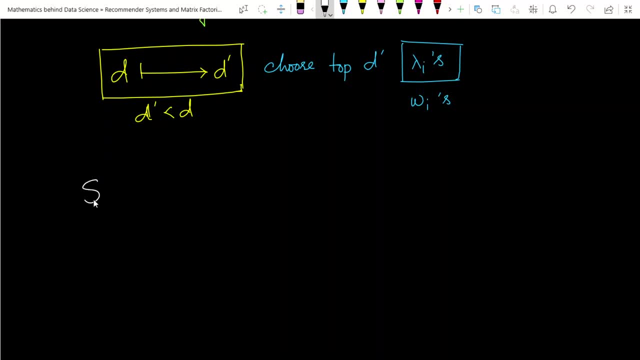 so the we have to actually doing the job. we have to find that eigenvalue and eigen vectors for the covariance matrix. so here, covariance matrix is s d cross d diamond one. so first we have to doing the matrix factorization for this covariance matter. so suppose, let we have to convert this: w is the lambda, capital lambda, and this is the w transpose. 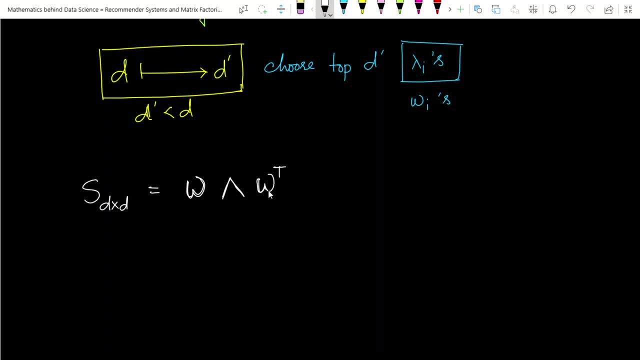 w transpose. w lambda w transpose. there is job that we have to do now. what will be the dimension of h vector? actually, these are the edge matrix. if you call these are the edge matrix, these are the edge matrix. okay, now what is will be the dimension for edge matrix? 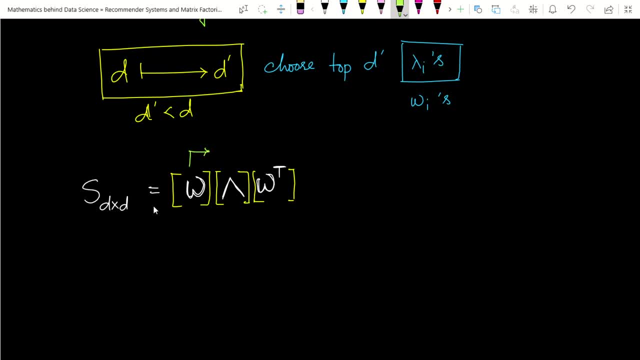 this dimension here. first, its dimensional will be so it start d to d, so its dimension will be d cross n. okay, sorry, sorry for that. d cross d. its dimension will be d cross d. similarly, its dimensional will be d cross d. okay, and now its dimensional will be. 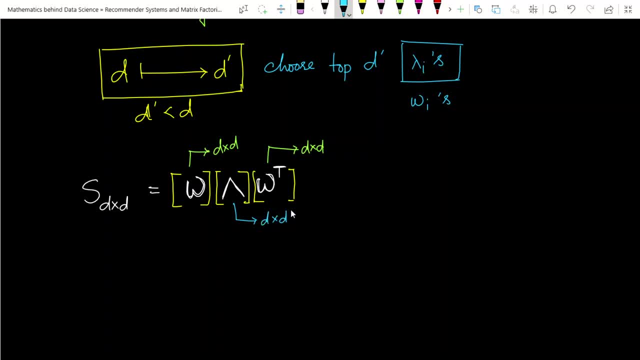 also d cross d edge matrix is square matrix. okay, these things are actually principal component analysis technique. these are the actually principal component. and w transport is the transpose matrix of this w. okay, now let's, what is the value? of h is matrix, what is it that we are setting? that is kind of an example of how to spread these matrix correct. our matrix is little bitgado, that is also collection, and then what we do, then we have to, by the way, and now let's for this matrix. we have a student, we have a second element, okay, and which is directly, directly on the other side of it. we are not going to use this point, however. 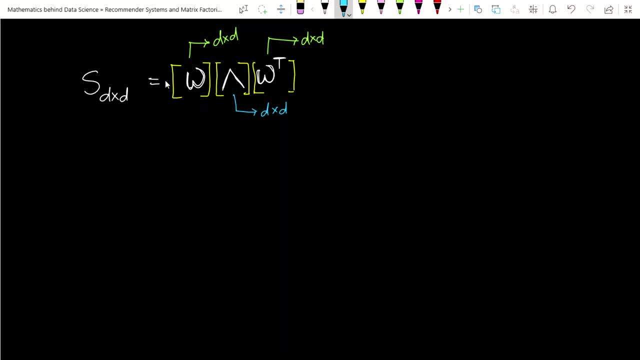 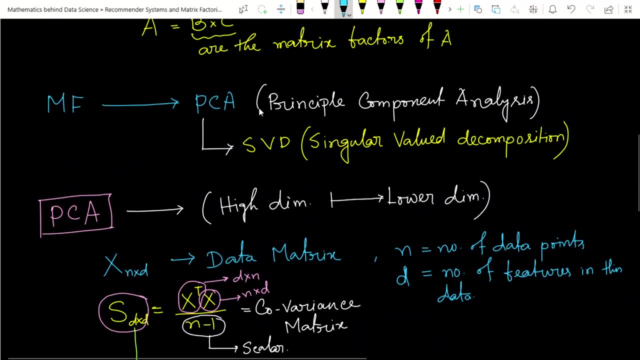 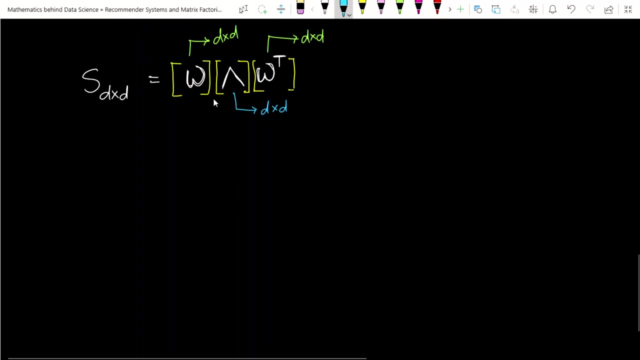 is w actually here? what is the w? this is the actually matrix factorization technique, that thing we have seen. these are the matrix factorization technique. these are the matrix factorization technique. okay, that's thing. so we'll see in future video how to doing this. but now let's try to connect that dots between factorizations and principal component. now what? 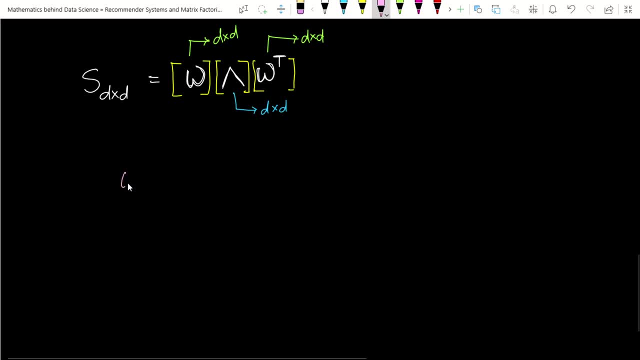 is the significant of this w, so w. here is a d d cross d dimensional vector. d cross d dimensional vector means, if you consider these things as a w1, small w1 means it is the suppose that it is the column vector, actually this column vector, of this capital w, let's say w2. 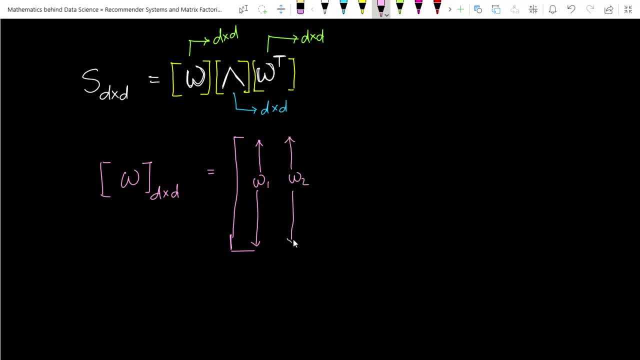 column vector. column vector. column vector- this is the w3 means column vector of the w. this is the column vectors of the w. okay, and as well it's the column vector wd, because it d cross d dimensional vector. okay, so this is the d cross d dimensional vector. 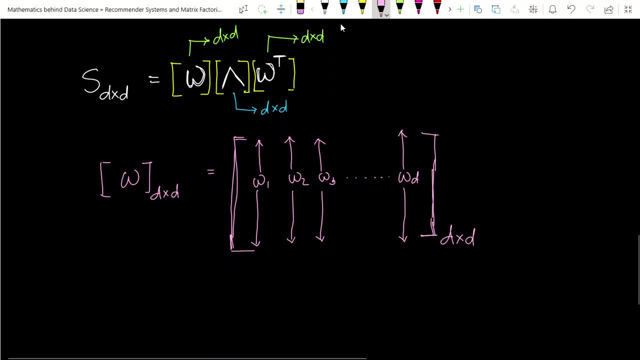 d cross d dimensional vector. d cross d dimensional vector, and these are the. these are the is and these are the. these are the is and these are the. these are the. is dimensional, is dimensional, it's dimensional. it is a column vector. it is a column vector, so its dimensional will be. 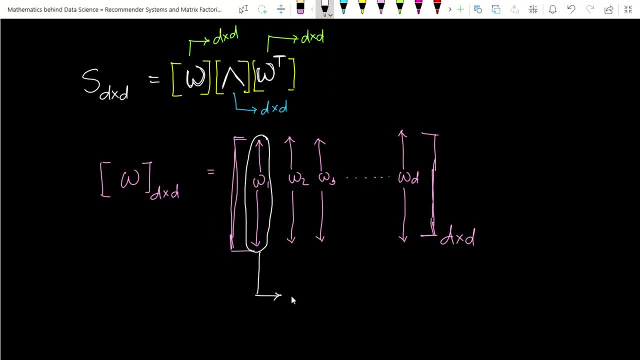 it is a column vector, so its dimensional will be: it is a column vector, so its dimensional will be: how much column single column first. how much column single column first. how much column single column first. how much rho d rho into single column? how much rho d rho into single column? 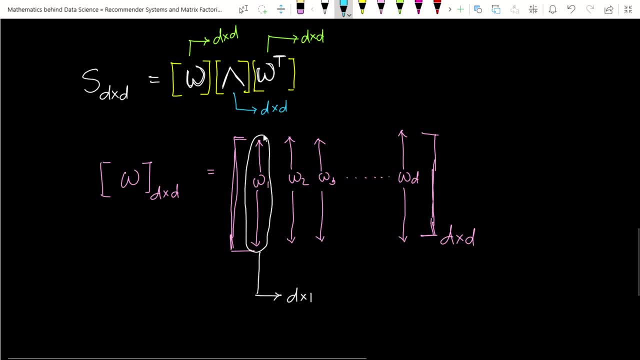 how much rho d rho into single column. this dimensional here, and these things are this dimensional here, and these things are this dimensional here, and these things are called the. these vectors called the. these vectors called the. these vectors actually called the. these are the actually called the. these are the. 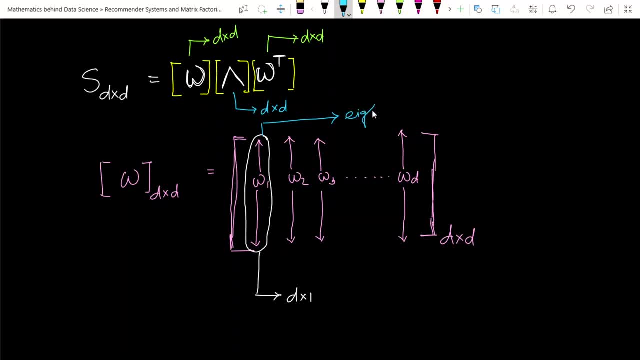 actually called the. these are the eigenvectors of, these are the eigenvectors of the set s, of the set s of the set s. this is called the eigenvectors. that is. this is called the eigenvectors. that is. this is called the eigenvectors. that is the main important. 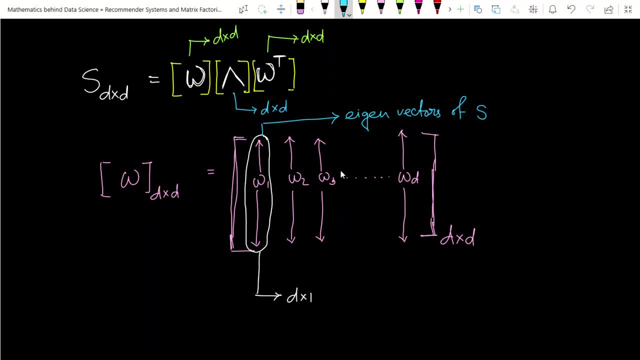 the main important, the main important. okay, these are the eigenvectors of it. okay, these are the eigenvectors of it. okay, these are the eigenvectors of it. now, let's now. let's now, let's see what is actually the lambda. let's see. 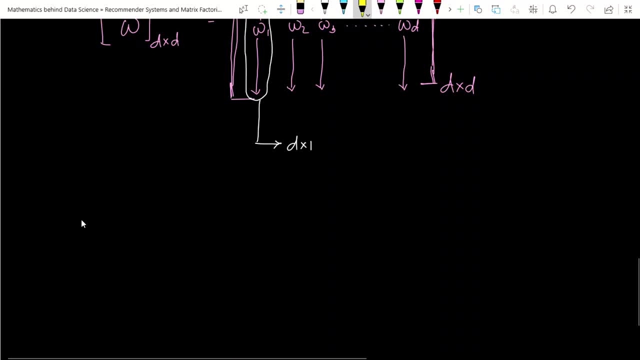 see what is actually the lambda. let's see, see what is actually the lambda, let's see it. see what is actually the lambda, let's see it. but teach this capital lambda, but teach this capital lambda, but teach this capital lambda. this is also a vector. this is sorry, this. 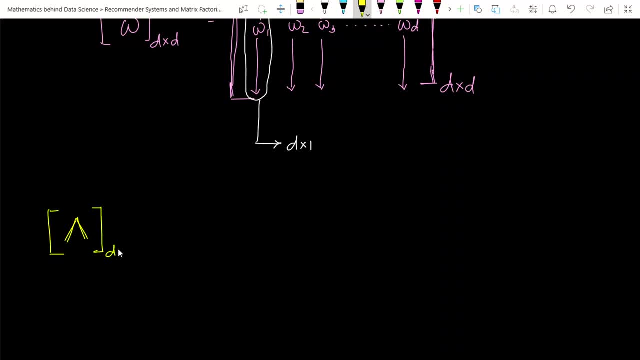 this is also a vector. this is sorry. this, this is also a vector. this is sorry. this is also a matrix- is also a matrix, is also a matrix, and the dimension of this matrix is d, and the dimension of this matrix is d, and the dimension of this matrix is d cross d. 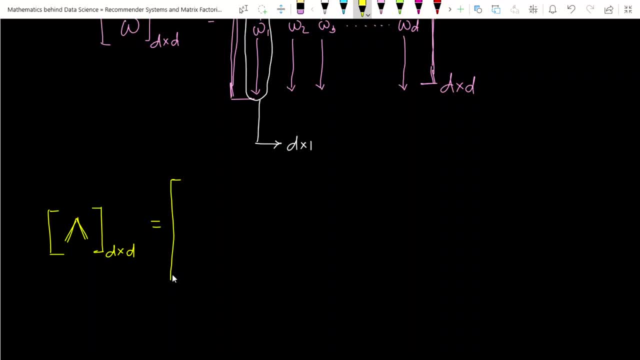 cross d, cross d, but this matrix is simple a, but this matrix is simple a, but this matrix is simple: a diagonal matrix, diagonal matrix, diagonal matrix, okay, so the diagonal value, the diagonal, okay, so the diagonal value, the diagonal. okay, so the diagonal value, the diagonal element of this element of this matrix. 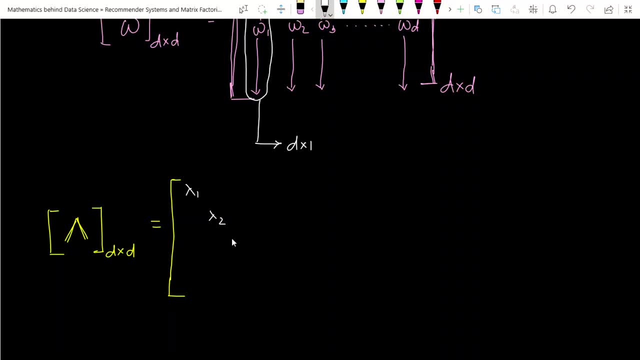 element of this element of this matrix. element of this element of this matrix is: lambda 1 small lambda 1. is lambda 1 small lambda 1 is lambda 1 small lambda 1. lambda 2, lambda 2 lambda 2 lambda d and rest of the null diagonal element is: 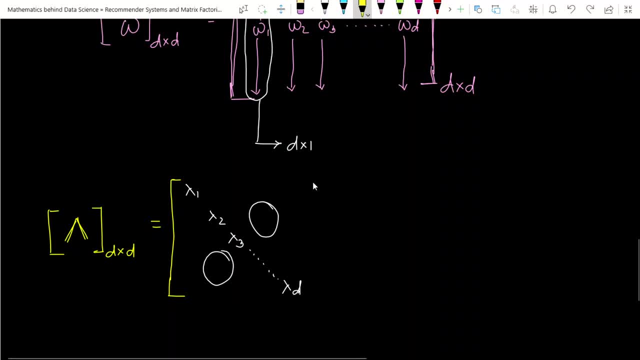 and rest of the null diagonal element is: and rest of the null diagonal element is zero, zero, zero. okay. rest of the null diagonal element: okay. rest of the null diagonal element: okay. rest of the null diagonal element is zero. these are the d cross d. these are the lambda 1, lambda 2, lambda 3. 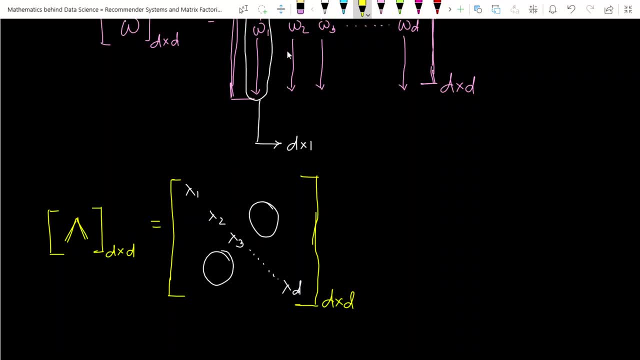 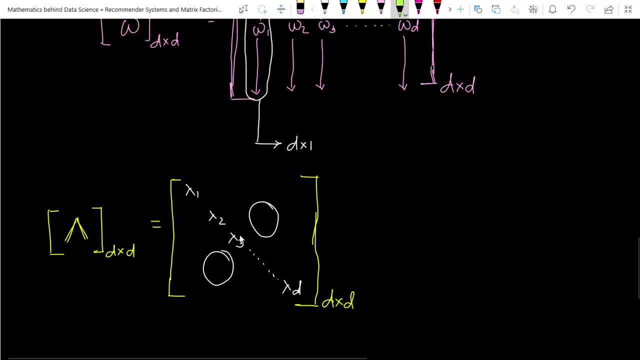 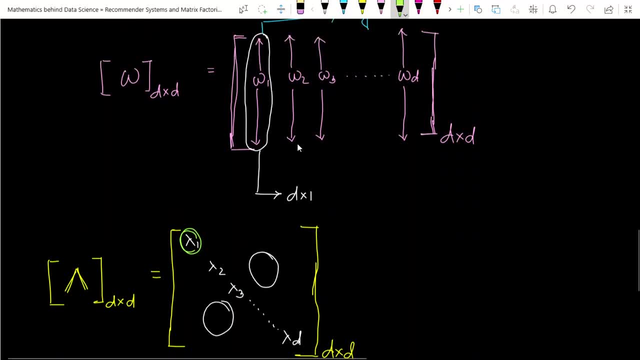 what here, lambda i is lambda i. here is the eigen values of s. these are the is the eigen values of s. these are the is the eigen values of s. these are the eigen vectors of s eigen vectors of s eigen vectors of s and corresponding. these are the eigen. 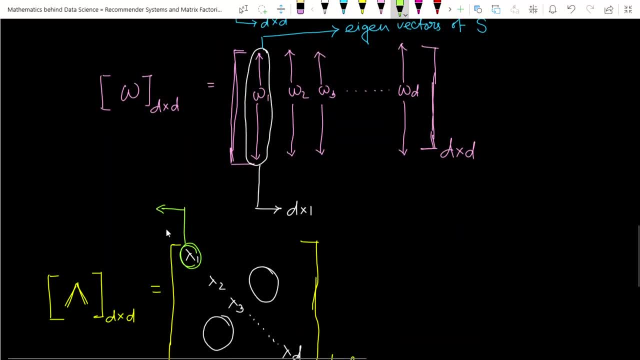 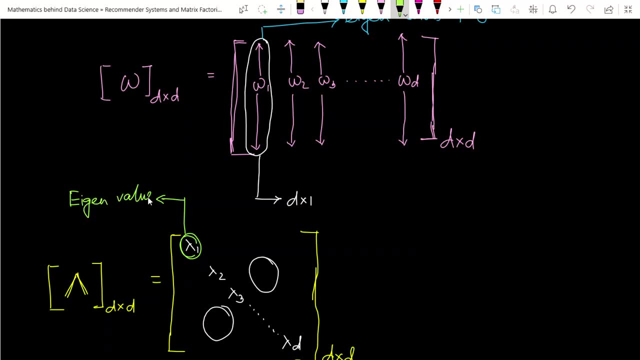 and corresponding. these are the eigen and corresponding, these are the eigen values of s values, of s values of s. this is the important, this is the important, this is the important. these are the called the eigen values. oh yes, oh yes, oh yes, i think you got the answer. 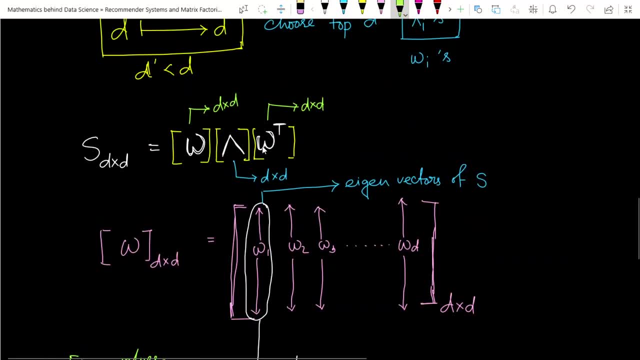 i think you got the answer. i think you got the answer. this, i think you got the answer. this is the important. by simply doing this is the important, by simply doing, this is the important. by simply doing this, matrix multiplication job, we can easily. matrix multiplication job, we can easily. matrix multiplication job. we can easily find what will be the matrix eigen value. find what will be the matrix eigen value. find what will be the matrix eigen value and what will be the eigenvector and what will be the eigenvector and what will be the eigenvector. that's the sample job you have to do. i. 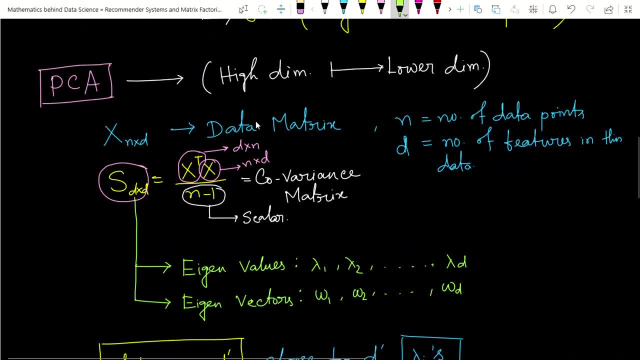 that's the sample job you have to do. i, that's the sample job you have to do. i think you got the answer. how this? think you got the answer, how this? think you got the answer, how this? matrix multiplications, matrix factorization. matrix multiplications, matrix factorization. 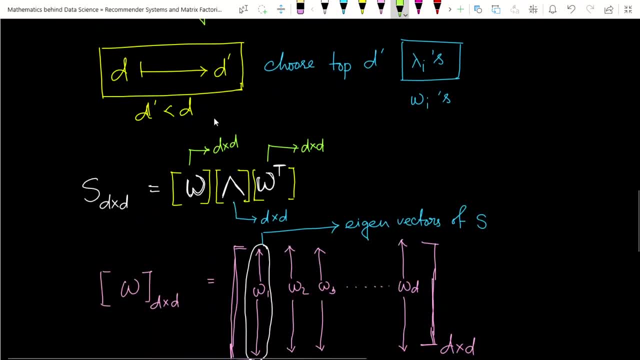 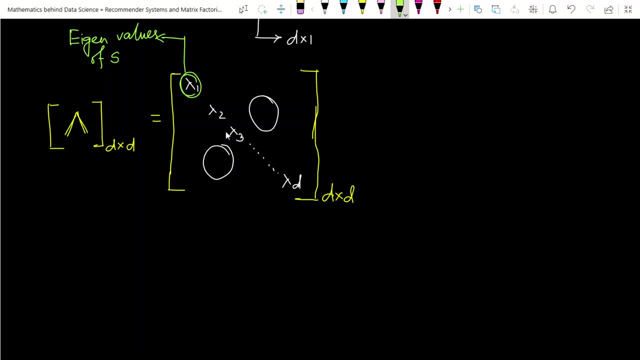 matrix multiplications, matrix factorization. techniques are important to find. techniques are important to find. techniques are important to find. this in pca: how it is important. you got this in pca. how it is important. you got this in pca. how it is important you got connected the dots between the matrix. 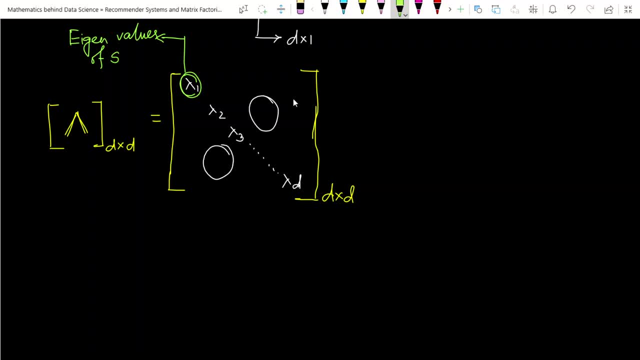 connected the dots between the matrix, connected the dots between the matrix factorizations and the pca factorizations and the pca factorizations and the pca. okay, now let's i, let's try to connect. okay, now let's i, let's try to connect. okay, now let's i, let's try to connect the singular value commission. 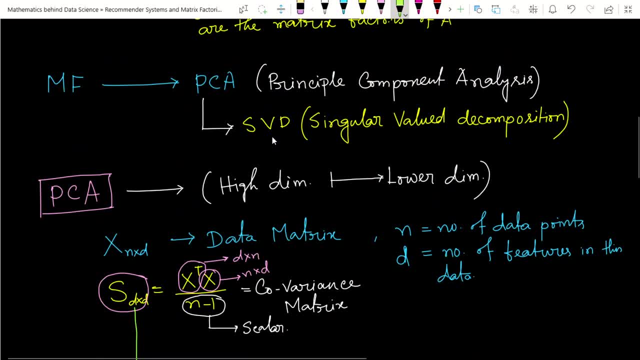 the singular value commission. the singular value commission, decomposition- what is this? let's try to decomposition. what is this? let's try to decomposition. what is this? let's try to understand it, understand it, understand it. what is singular value decomposition? what is singular value decomposition? what is singular value decomposition technique? 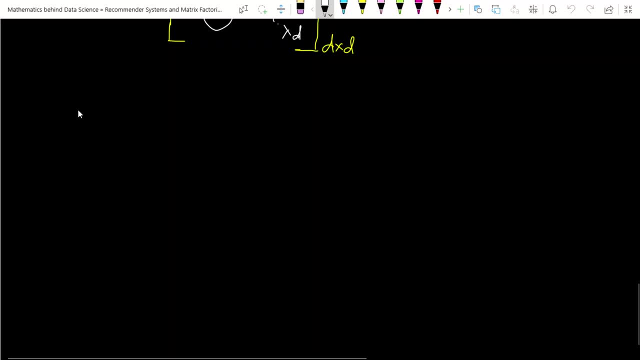 technique, technique. now, let's try to connect the dots now. let's try to connect the dots now. let's try to connect the dots between the matrix factorizations and between the matrix factorizations, and between the matrix factorizations and singular value decompositions problem. singular value decompositions problem. 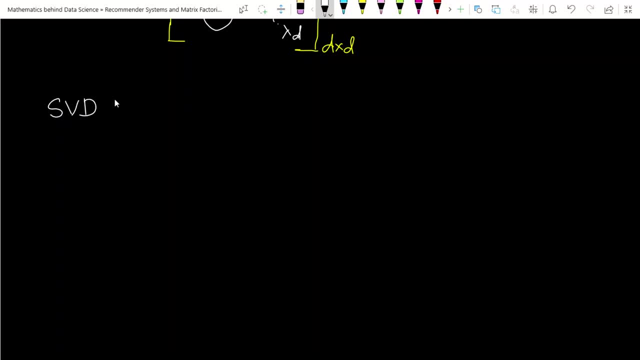 singular value decompositions problem. what is this singular value decomposition? what is this singular value decomposition? what is this singular value decomposition? what is this technique? the full name of what is this technique? the full name of what is this technique, the full name of this is singular value decomposition. 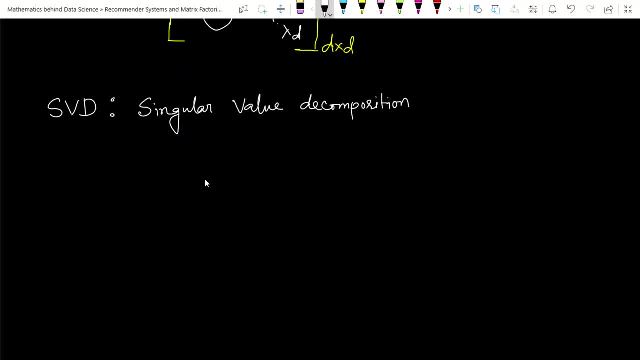 singular value decompositions. what is this singular value decompositions? what is this singular value decompositions? what is this? let's try to connect it, let's try to connect it, let's try to connect it. so this, this technique, the. so this, this technique, the. so this, this technique, the singular value decomposition. 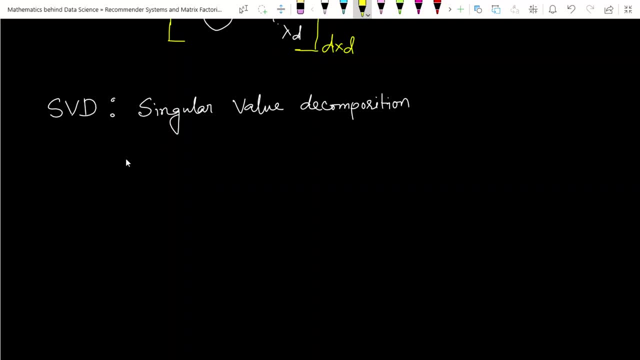 singular value decomposition. singular value decomposition is a simple technique of the matrix, is a simple technique of the matrix, is a simple technique of the matrix: factorization technique, factorization technique, factorization technique. if the sample a matrix factorization, if the sample a matrix factorization, if the sample a matrix factorization technique. that's related. 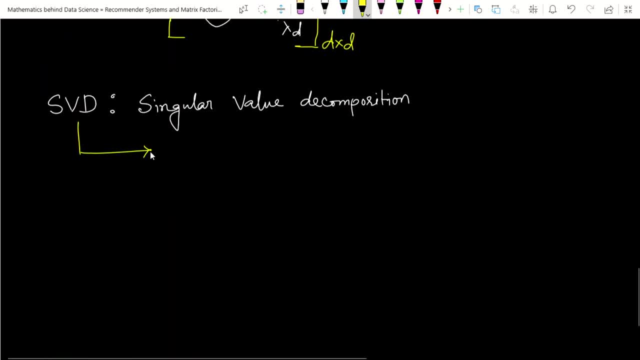 technique that's related. technique that's related. that's also related to this principal. that's also related to this principal. that's also related to this principal. component analysis, component analysis, component analysis: it's a matrix factorization technique, technique that is related to the principal component, the principal component analysis technique. okay, 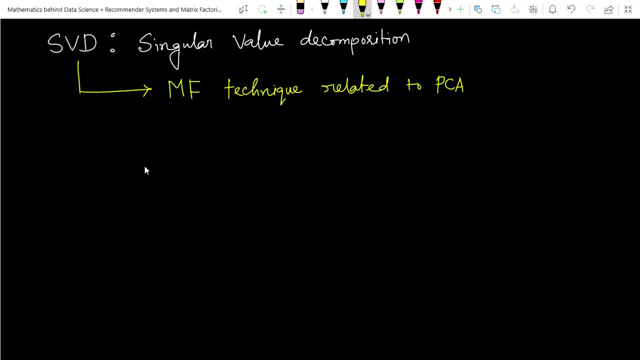 the principal component analysis technique. okay, the principal component analysis technique. okay, it's related to the principal component. let's it's related to the principal component. let's, it's related to the principal component. let's see, understand, let's see, see, understand, let's see, see, understand, let's see. so the principal component analysis in. 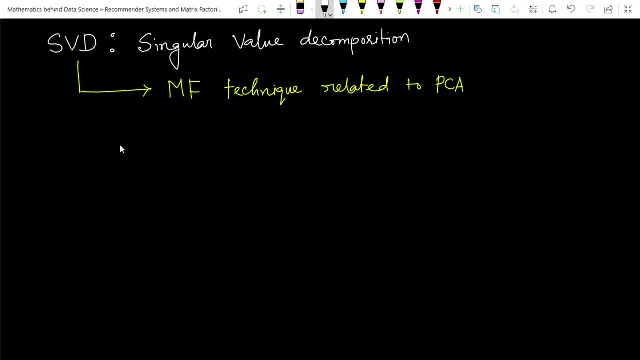 so the principal component analysis in. so the principal component analysis in principal component analysis. principal component analysis in principal component analysis. principal component analysis in principal component analysis. principal component analysis, principal component analysis. so first compare it to the principal. so first compare it to the principal. so first compare it to the principal component analysis to the sbud. 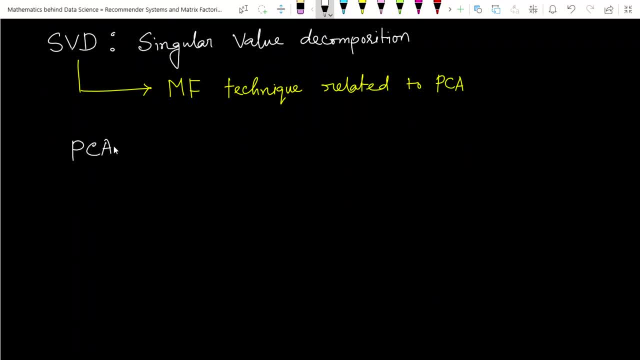 component analysis to the sbud. component analysis to the sbud. so in principal component analysis, the. so in principal component analysis, the. so in principal component analysis, the matrix that we have used in the matrix, that we have used in the matrix that we have used in the principal component analysis, the matrix. 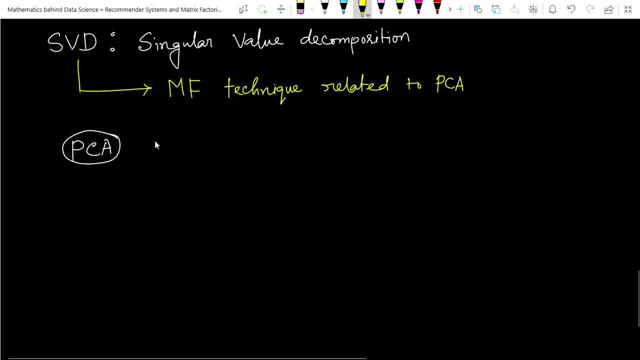 principal component analysis. the matrix, principal component analysis, the matrix that we have used. this matrix is that we have used? this matrix is that we have used? this matrix? is s that we have used? if you, just if you s that we have used? if you just if you. 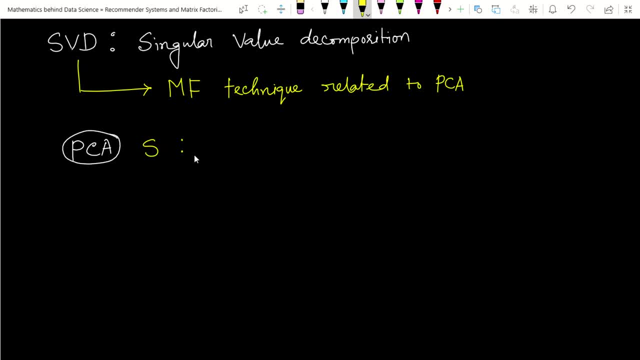 s that we have used. if you, just, if you just try to remember the characteristics, just try to remember the characteristics, just try to remember the characteristics of this matrix is a square matrix first of this matrix is a square matrix first of this. matrix is a square matrix first, first it must be a square matrix. and as 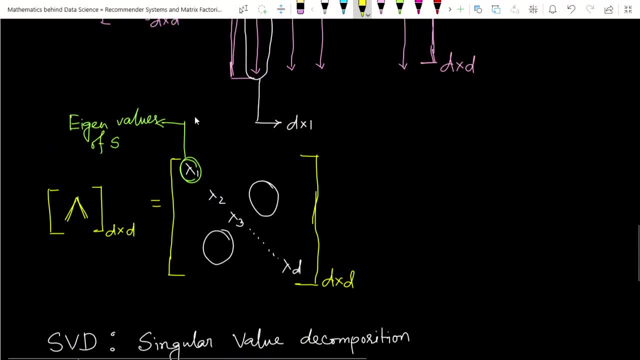 first it must be a square matrix and as first it must be a square matrix, and as well, it's a symmetric matrix. well, it's a symmetric matrix. well, it's a symmetric matrix. okay, because we have to actually just okay, because we have to actually just okay, because we have to actually just try to see that. 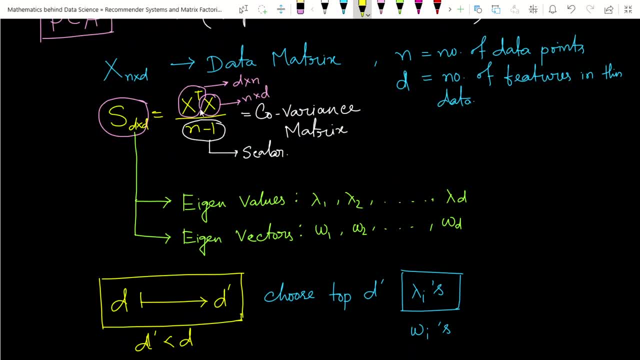 actually it is the multiplications of two terms. actually it is the multiplications of two terms. actually it is the multiplications of two terms. a single x data matrix: it's the. a single x data matrix: it's the. a single x data matrix: it's the multiplication of a data matrix. 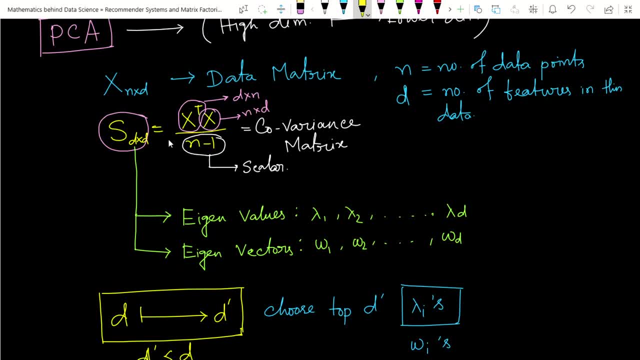 multiplication of a data matrix. multiplication of a data matrix: x transpose x. so, because of this, we got x transpose x. so, because of this, we got x transpose x. so, because of this, we got this square matrix, this square matrix, this square matrix, and and must be, since we have multiplying. 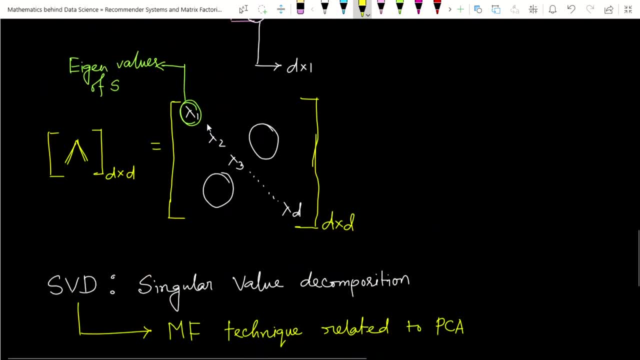 and and must be, since we have multiplying and and must be, since we have multiplying this, this, this transformation to x is must be a transformation to x, is must be a transformation to x, is must be a symmetric matrix, symmetric matrix, symmetric matrix. okay, that is the first characteristics. it's: 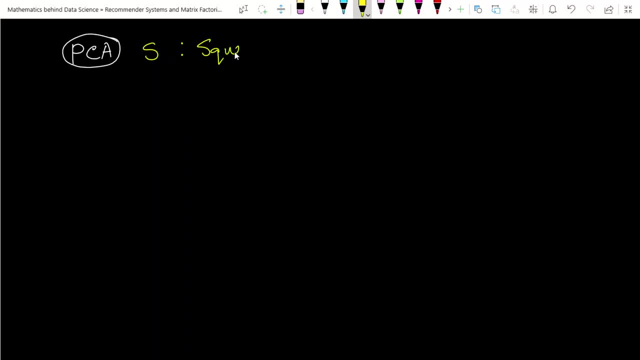 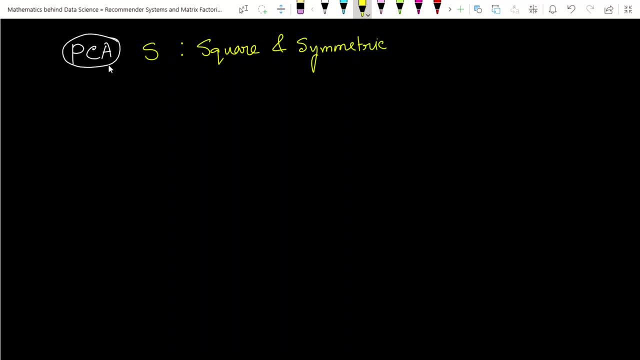 this must be a symmetric matrix. okay, this must be a symmetric matrix. okay, this must be a symmetric matrix. okay, that is the principal component analysis. that is the principal component analysis. that is the principal component analysis. that the x, that the x, that the x, but in a, in svd, in singular decomposition. 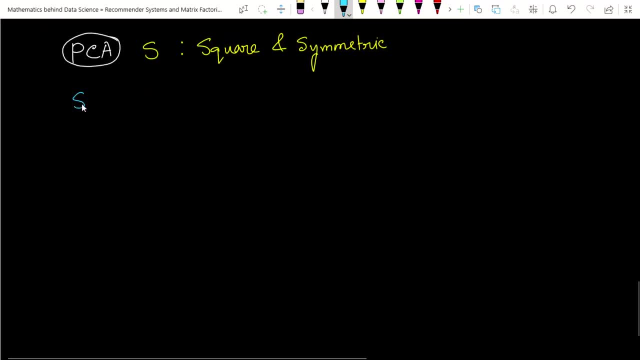 but in a in svd in singular decomposition, but in a in svd in singular decomposition. singular singular value. decompositions in singular singular value. decompositions in singular singular value. decompositions in svd: the matrix svd. the matrix svd. the matrix svd. svd. the matrix svd. the matrix svd. 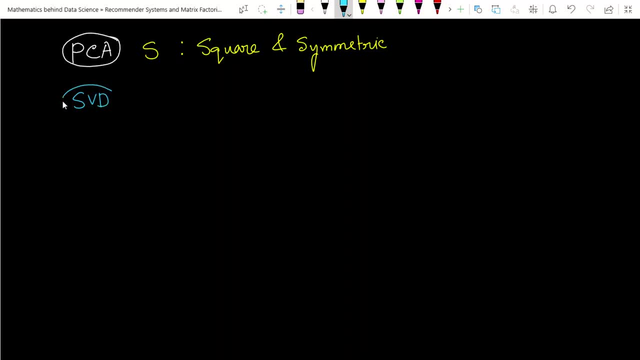 svd the matrix, svd the matrix. svd the matrix that we are going to use. it's a the matrix that we are going to use. it's a the matrix that we are going to use. it's a rectangular matrix, rectangular matrix, rectangular matrix, simple. it is a rectangular matrix x, not. 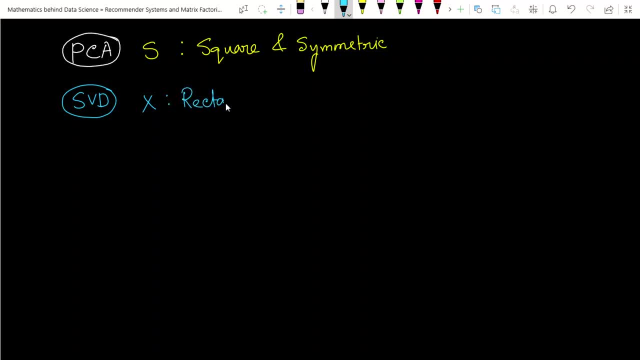 simple. it is a rectangular matrix x, not simple. it is a rectangular matrix x, not it's any matrix, it's any rectangular. it's any rectangular matrix that we have. it's any rectangular matrix that we have. it's any rectangular matrix that we have used, used, used, okay. so here any. so its dimension will. 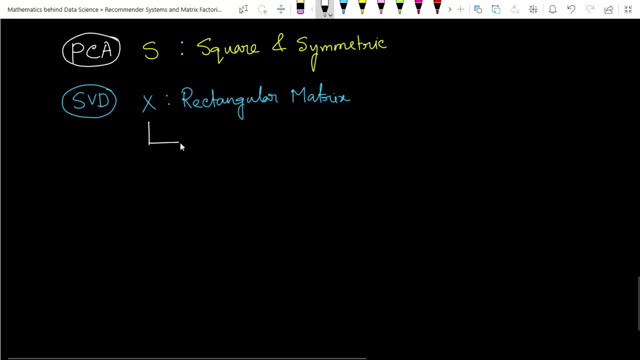 okay, so here any, so its dimension will okay. so here any, so its dimension will be. let, let be let. let be, let let. for simplicity, it's for simplicity, it's for simplicity, it's let it dimension is encrusted, let it, dimension is encrusted. 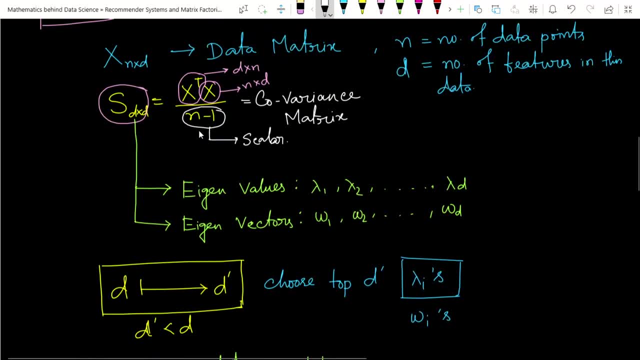 let it dimension is encrusted- that we have some means, simply a data. that we have some means, simply a data. that we have some means, simply a data matrix act. you can treat these as a matrix act. you can treat these as a matrix act. you can treat these as a simple data matrix. okay. 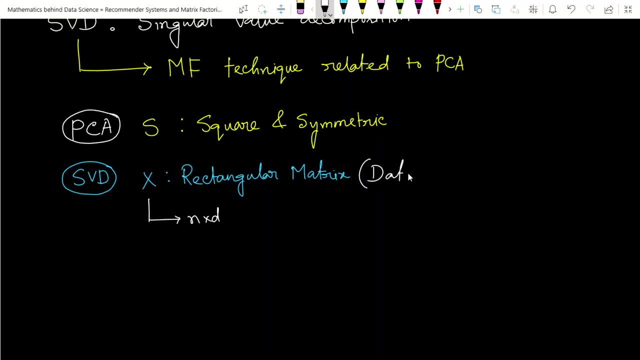 simple data matrix. okay, simple data matrix. okay, these things are the simple data matrix. these things are the simple data matrix. these things are the simple data matrix. another way: this is a simple data matrix. x, x is a simple data matrix. okay, now let's try to understand this. 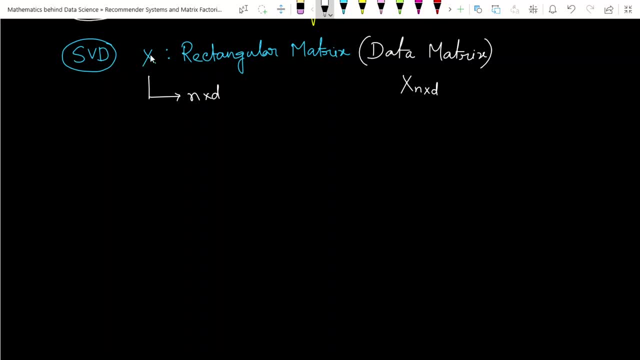 is a simple data matrix. okay, now let's try to understand. this is a simple data matrix. okay, now let's try to understand this: sbt this x. how to sbt this x. how to sbt this x. how to how to the matrix factorization technique. 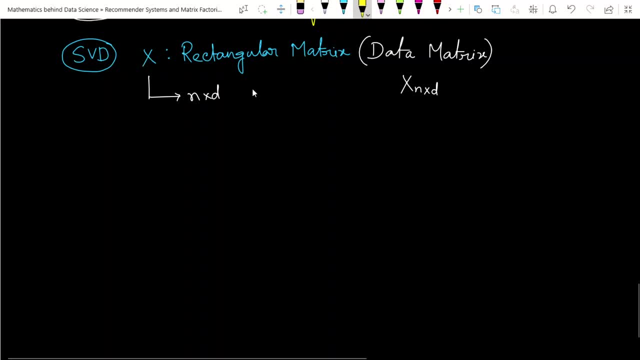 how to the matrix factorization technique, how to the matrix factorization technique, how these things are important in how these things are important in how these things are important in sbt technique. let's see so, the matrix that sbt technique. let's see so, the matrix that. 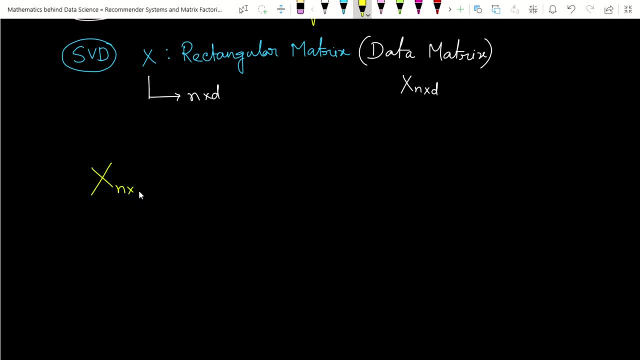 sbt technique, let's see. so the matrix that we have, we have, we have: x, it's the simple n cross g. matrix, x, it's the simple n cross g. matrix, x, it's the simple n cross g matrix, ordered matrix, ordered matrix, ordered matrix. and the first thing that we have to 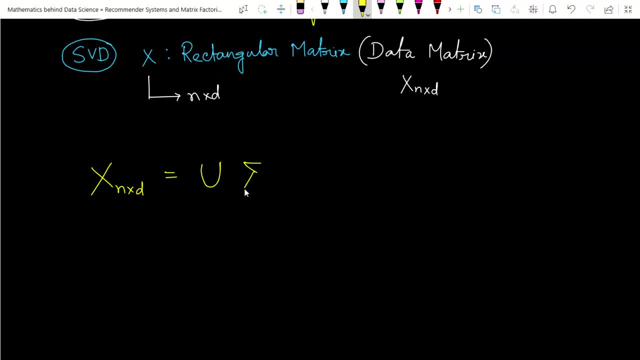 and the first thing that we have to, and the first thing that we have to convert it. say u it's sigma, we have to convert it. say u it's sigma, we have to convert it. say u it's sigma. we have to decompose like that: and it's v transpose. 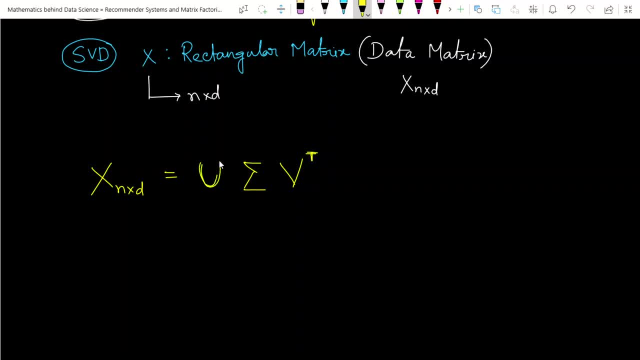 decompose, like that and it's v transpose. decompose, like that and it's v transpose, v transpose. that is the decomposition, v transpose. that is the decomposition, v transpose. that is the decomposition. that is the factorizations we have to. that is the factorizations we have to. 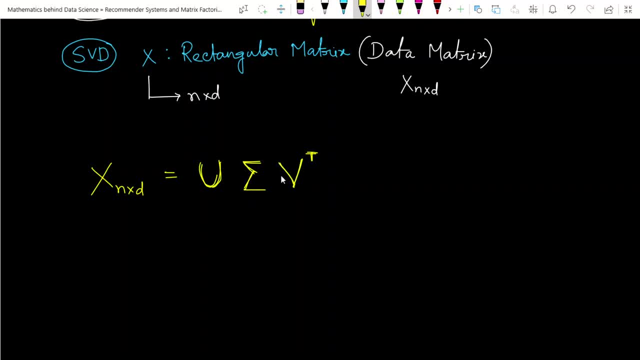 that is, the factorizations we have to do. that is that now let's try to connect the. that is that now let's try to connect the. that is that now let's try to connect the dots, these matrix factorizations, dots these matrix factorizations, dots these matrix factorizations to the. these matrix, how, this matrix, how. 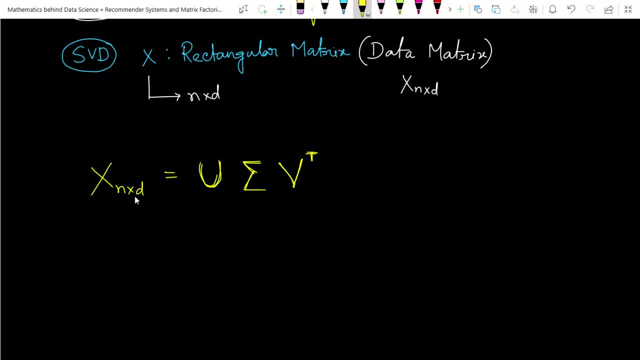 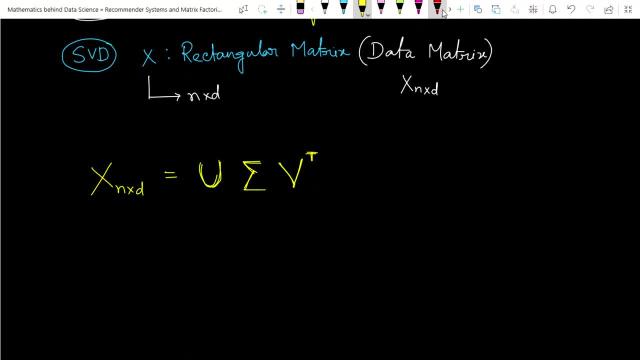 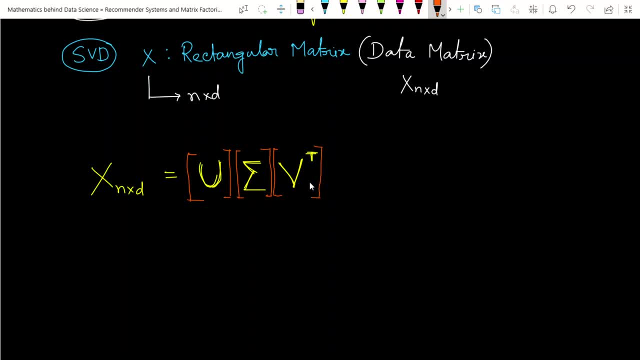 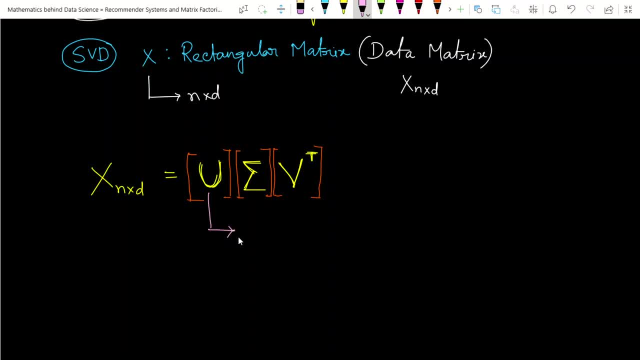 understand it. what will be the dimension of u, of u, of u? what will be the dimension of? what will be the dimension of u? what will be the dimension of u? what will be the dimension of u? u the dimension of u will be here, so u, the dimension of u will be here, so 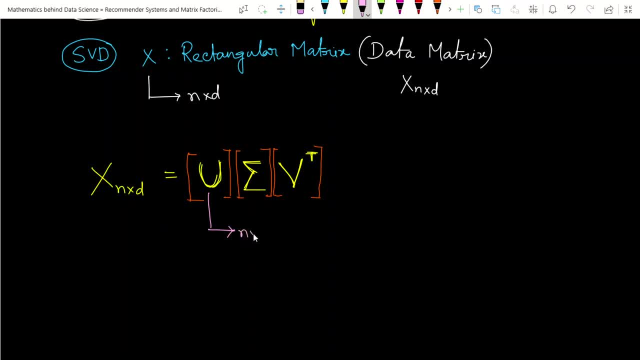 u, the dimension of u will be here, so first. it is starting from n, so must be first it is starting from n, so must be first. it is starting from n, so must be. it is a square matrix, n cross n. it is a square matrix, n cross n. 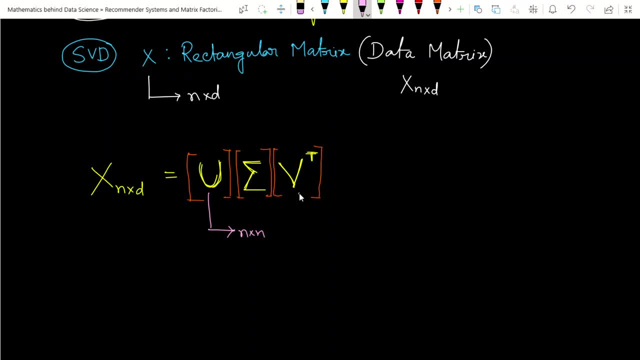 it is a square matrix: n cross n, and it's end with d, so dimension of the, and it's end with d, so dimension of the, and it's end with d, so dimension of the. v will be, v will be v will be d cross d, d cross d. 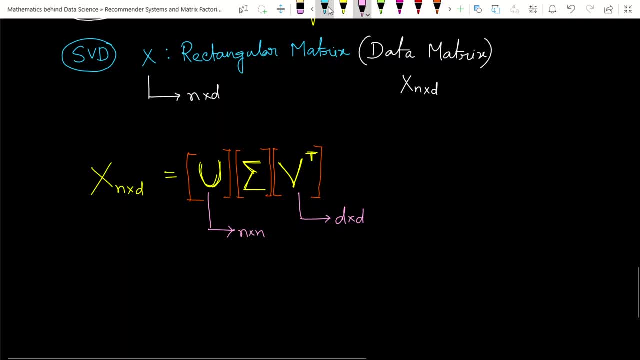 d, cross d. now, based on this dimension of the, now, based on this dimension of the, now, based on this dimension of the sigma, these sigma, these sigma, these, these things are called the sigma, these things are called the sigma, these things are called the sigma regulator, sigma, regulator, sigma. 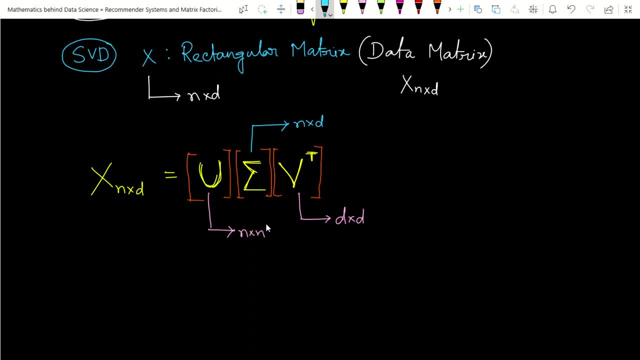 regulator sigma. so because these regions, it is canceled. so because these regions it is canceled. so because these regions, it is canceled out this and this and cancel out this, out this and this, and cancel out this, out this and this and cancel out this, it is canceled so. 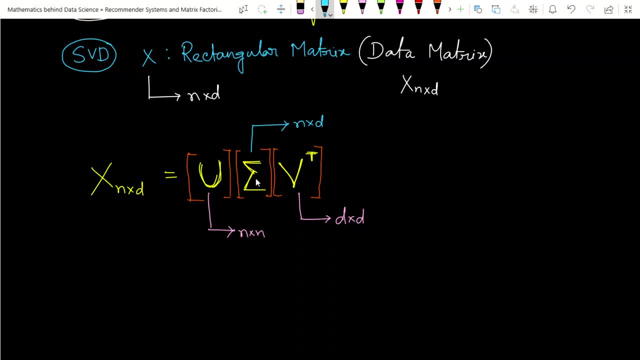 it is canceled, so it is canceled. so matrix multiplication is possible here. matrix multiplication is possible here. matrix multiplication is possible here. these are the simple day definitions now. these are the simple day definitions now. these are the simple day definitions now. these matrix are called the these. these matrix are called the these. 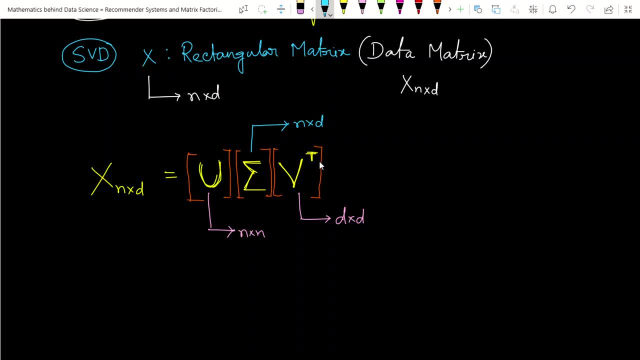 these matrix are called the. these matrix, the right side, this matrix is matrix the right side. this matrix is matrix the right side. this matrix is called the right singular valued, called the right singular valued, called the right singular valued matrix of matrix, of matrix of x, x, x. this matrix is called the. 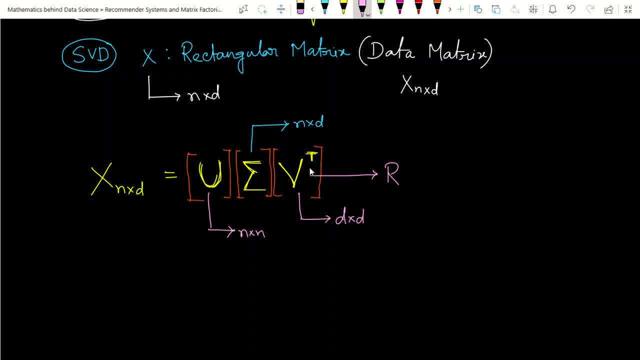 this matrix is called the. this matrix is called the right singular valued matrix. we'll see right singular valued matrix. we'll see right singular valued matrix. we'll see how these matrix are important in our how. these matrix are important in our how. these matrix are important in our computation. we'll say this thing, but 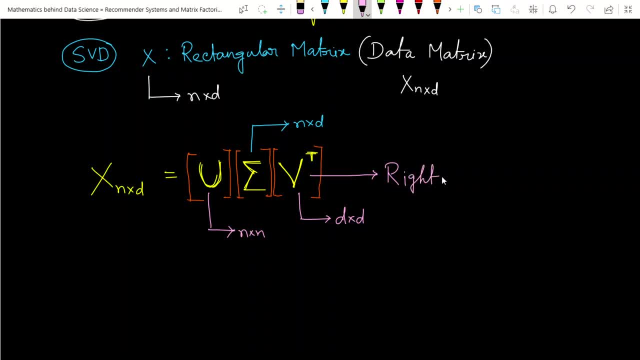 computation, we'll say this thing. but computation, we'll say this thing. but this matrix is called. this matrix is called. this matrix is called right, singular right, singular vectors of right, singular vectors of right, singular vectors of, of x, and this matrix, and this matrix, and this matrix is called the. 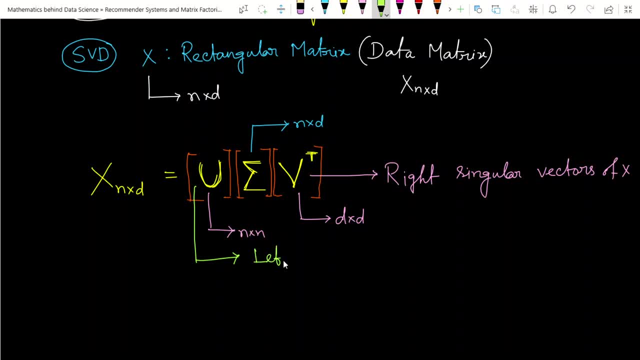 left. singular. vectors of x. this mat, this matrix u is called the. this mat, this matrix u is called the. this mat, this matrix u is called the left and this r is called the right left and this r is called the right left and this r is called the right singular. 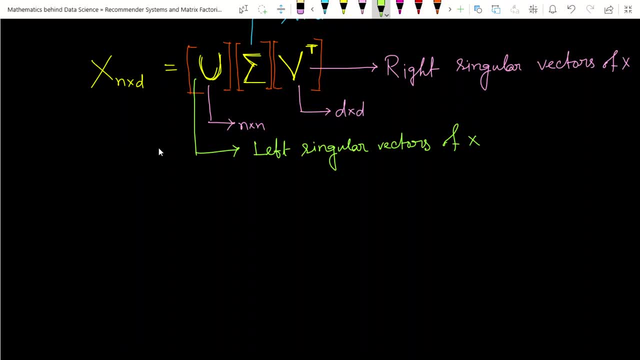 singular. singular. okay now, uh, just try to compare this. okay now, uh, just try to compare this. okay now, uh, just try to compare this thing to the thing, to the thing, to the pca: principal component analysis in pca. pca: principal component analysis in pca. pca: principal component analysis in pca. we have seen this. instead of using x, we. 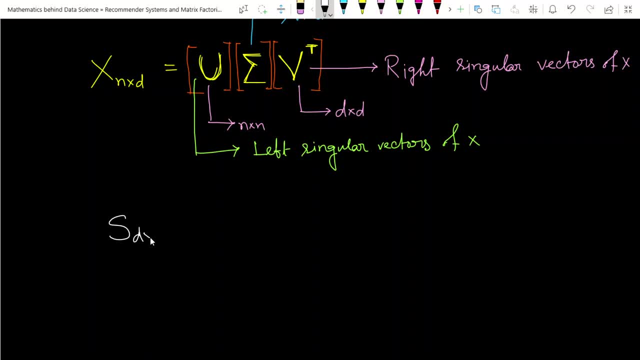 we have seen this instead of using x. we we have seen this. instead of using x, we have used here the covariance vector. have used here the covariance vector. have used here the covariance vector. covariance matrix x- cross d. covariance matrix x- cross d. covariance matrix x- cross d. and we will decompose into like that: 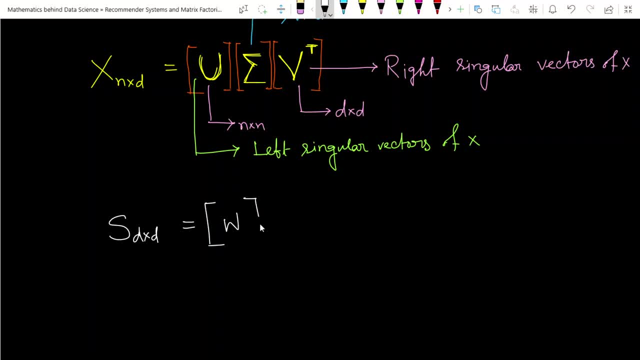 and we will decompose into like that and we will decompose into like that: the first one is the first one is the first, one is w and the second and the second. and the second matrix is the matrix is, the matrix is the capital lambda and the third matrix is: 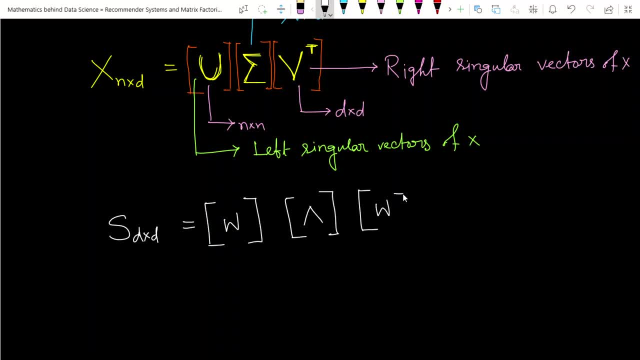 capital lambda and the third matrix is capital lambda and the third matrix is the w transpose, since it's the square matrix, since it is, since it's the square matrix, since it is, since it's the square matrix, since it is square matrix, so h dimensional must be. 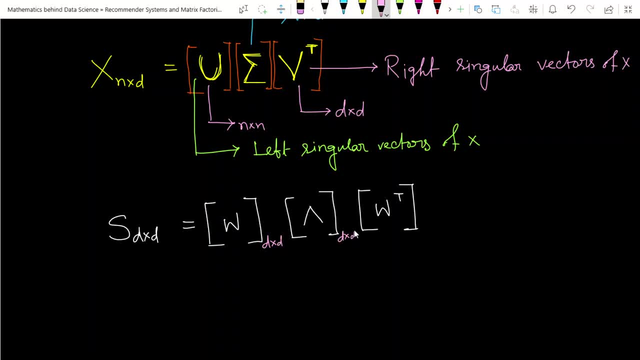 square matrix, so h dimensional must be square matrix, so h dimensional must be the square data is the square data is the square data is d cross d, d cross d, d cross d. this is also d cross d. this is also d cross d. this is also d cross d. okay, that we have seen. 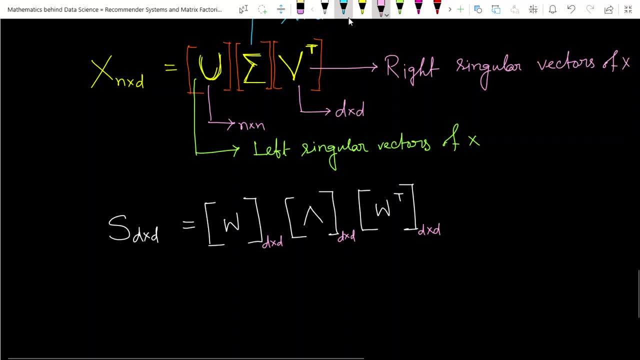 okay that we have seen, okay that we have seen. so now this w. what is the importance of so now, this w. what is the importance of so now this w. what is the importance of w here and what it just try to compare w here and what it just try to compare? 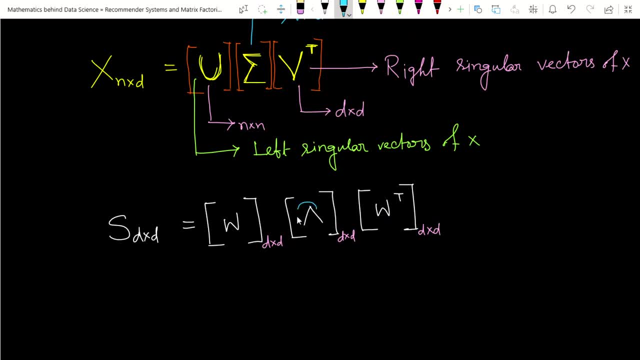 w here and what it. just try to compare it side by side. i think it will look it side by side. i think it will look it side by side. i think it will look. is lambda, it's give the role of to find. is lambda, it's give the role of to find. 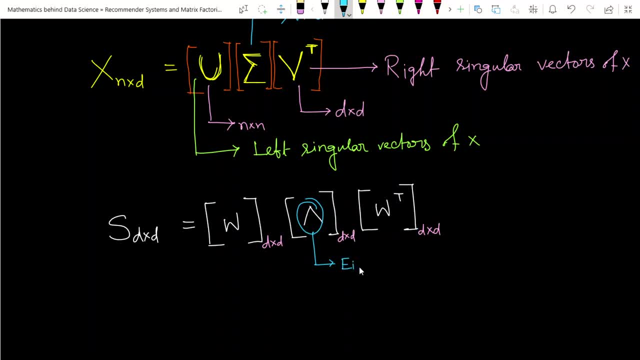 is lambda. it's give the role of to find the eigenvalues of x, eigenvalues of s. this w, eigenvalues of s this w, eigenvalues of s. this w and this w are given the role to find and this w are given the role to find. 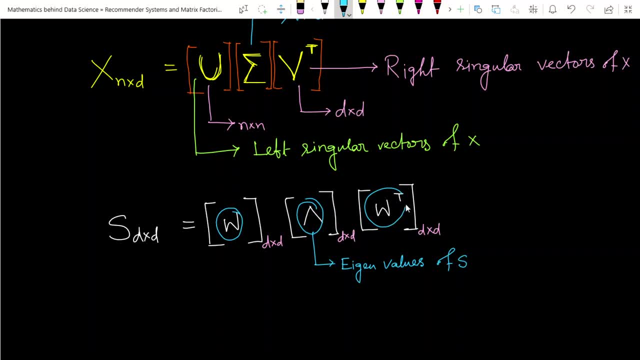 and this: w are given the role to find the eigenvectors of x. the eigenvectors of x, the eigenvectors of x. given the role to find the eigenvectors. given the role to find the eigenvectors. given the role to find the eigenvectors. 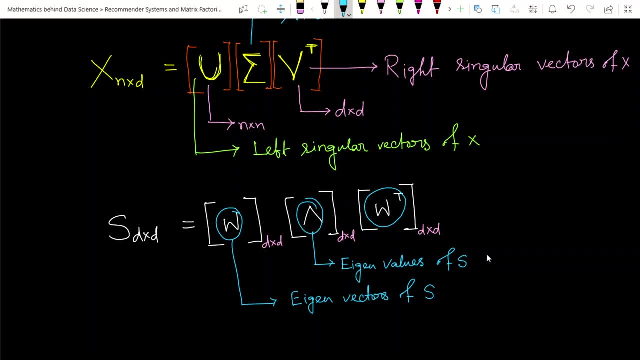 eigenvectors, eigenvectors, eigenvectors of s. okay, we have already seen of s. okay, we have already seen of s. okay, we have already seen this, and these things are called actually this, and these things are called actually this, and these things are called actually pca. 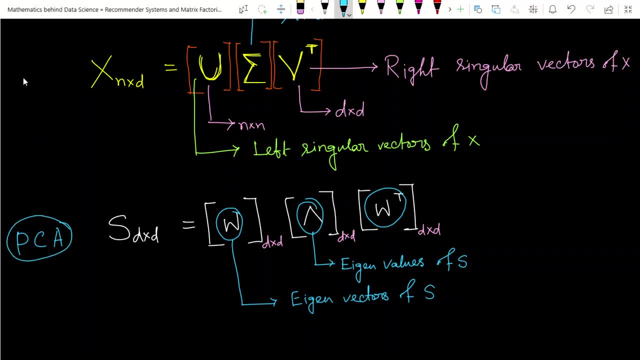 pca, pca. these are the pca technique we got, we have. these are the pca technique we got, we have. these are the pca technique we got. we have seen, and this is the singular value: sbt seen and this is the singular value sbt seen and this is the singular value: sbt. okay, now let's try to compare this side. 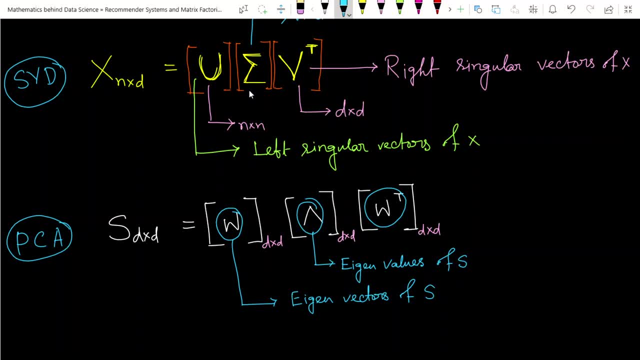 okay, now let's try to compare this side. okay, now let's try to compare this side by side by side by side. what is the significant here? sigma here. what is the significant here, sigma here. what is the significant here, sigma here- actually middle value. give the actually middle value. give the. 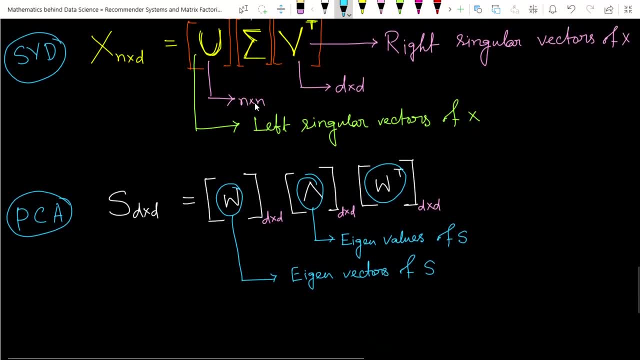 actually middle value. give the eigenvalues here, the same kinds of things. eigenvalues here, the same kinds of things. eigenvalues here, the same kinds of things also. we will got from this sigma also. we will got from this sigma also. we will got from this sigma. uh, this is sorry, this is the. this is. 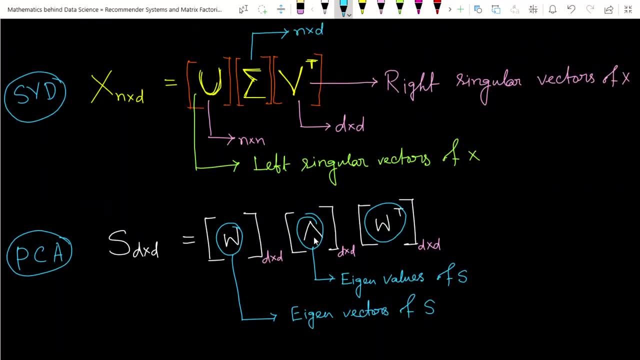 uh, this is sorry. this is the. this is. uh, this is sorry, this is the. this is capital. this is sigma and this is the capital. this is sigma and this is the capital. this is sigma and this is the capital lambda three. capital lambda is. capital lambda three. capital lambda is: 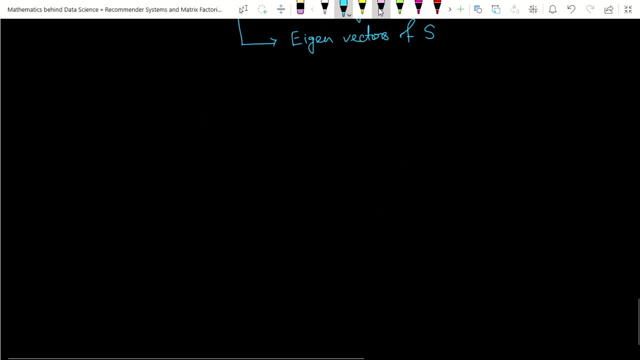 capital lambda three. capital lambda is the capital c, the capital c, the capital c. okay, okay, okay, so the capital sigma, so the capital sigma, so the capital sigma, the dimension of the capital sigma in sbd. the dimension of the capital sigma in sbd, the dimension of the capital sigma in sbd dimensionally: what is a dimensional is? 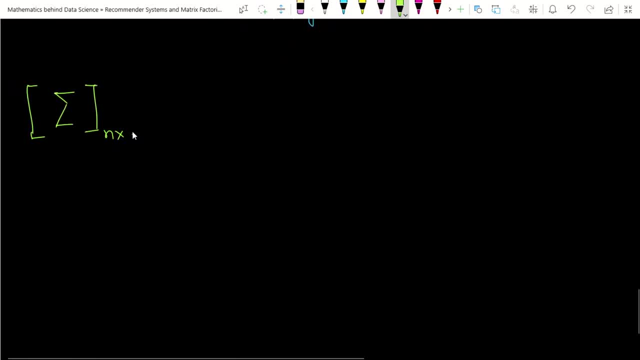 dimensionally, what is a dimensional is. dimensionally, what is a dimensional is n cross d. the dimension is n cross d, n cross d. the dimension is n cross d, n cross d. the dimension is n cross d. yeah, this matrix actually will be look. yeah, this matrix actually will be look. 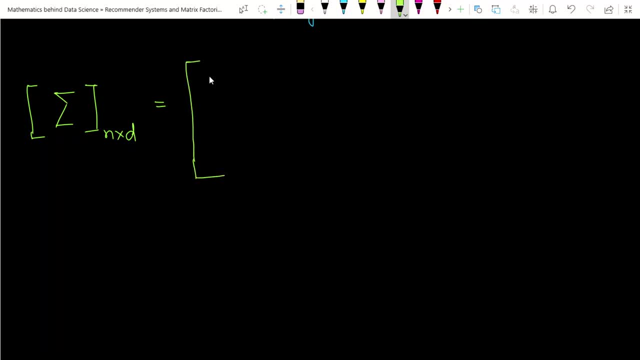 yeah, this matrix actually will be look like like, like this type of this type of this type of since, since, since here we have how much row n rows and here we have how much row n rows and here we have how much row n rows and d column. 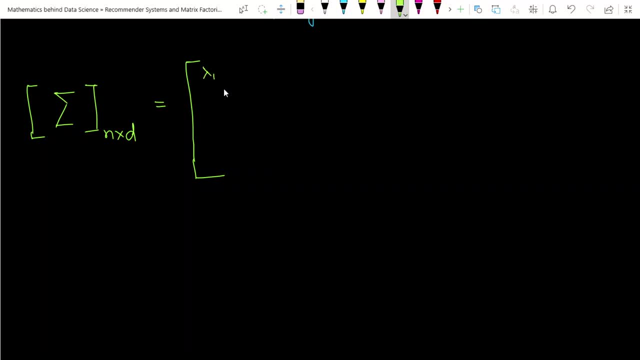 d column, d column, so the, or so the, or so the, or lambda one, lambda one, lambda one. sorry, here i'm taking the diagonal, sorry, here i'm taking the diagonal, sorry, here i'm taking the diagonal element. as like this element, as like this element, as like this: s1, small, s1, small, s2. 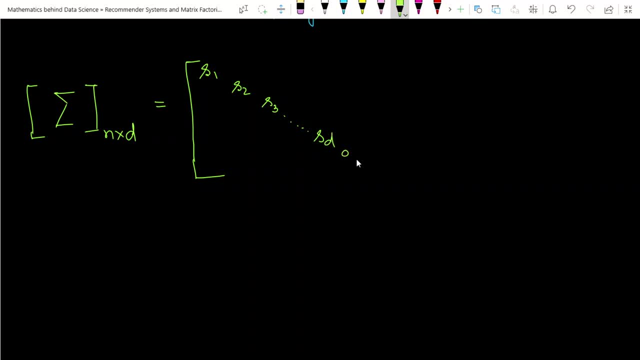 small s small s small s d and rest of the zeros, rest of the elements are the zeros. this is the n cross d and here must be. this is the n cross d and here must be. this is the n cross d and here must be. n must be less than the dimension. 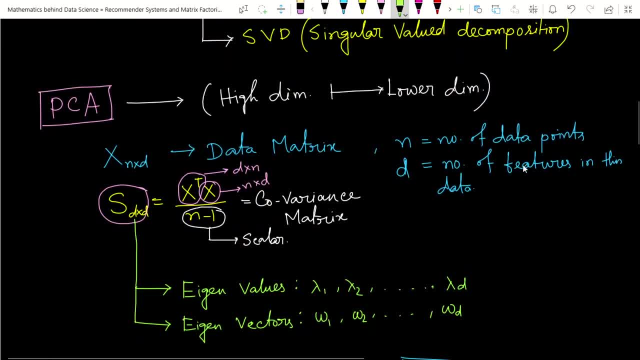 n must be less than the dimension. n must be less than the dimension. say this data actually here the number. say this data actually here the number. say this data actually here the number of data points and ad is the must be of data points and ad is the must be. 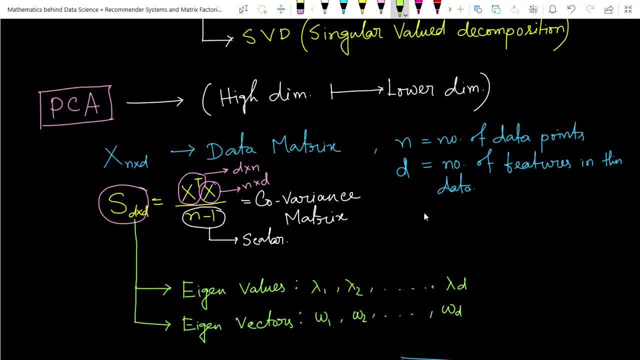 of data points and ad is the must be the number of data features vector. the number of data features vector, the number of data features vector. here d must be, here d must be here, d must be maybe equal, or maybe equal, or maybe equal, or like that. like this kind of vectors, we 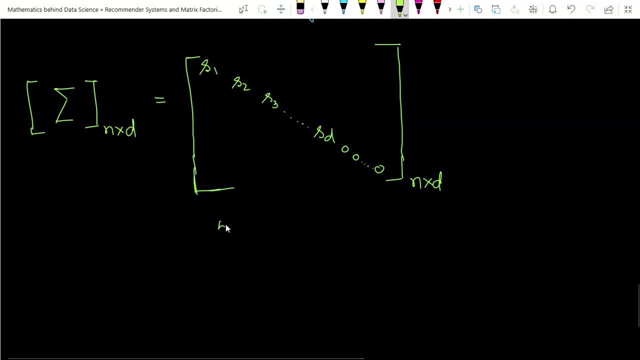 like that, like this kind of vectors, we like that, like this kind of vectors, we will got, will got, will got. okay, okay, okay. when the d is, when the d is, when the d is less than equals to m, less than equals to m, less than equals to m- if this thing happened, then we got this. 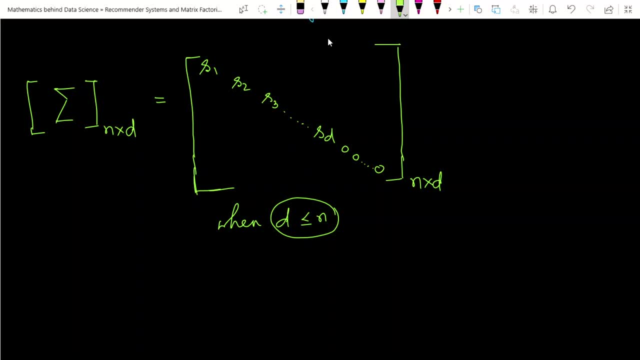 if this thing happened, then we got this. if this thing happened, then we got this kind of rectangular matrix. so here, this kind of rectangular matrix. so here, this kind of rectangular matrix. so here, this s one that we got. the s i is is a. i s one that we got. the s i is is a i. 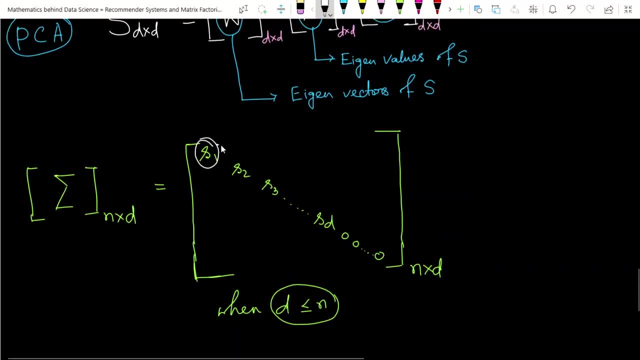 s one that we got. the s i is is a i that give the role. it is the singular that give the role. it is the singular that give the role. it is the singular. values, of values, of values, of these values are called the singular. these values are called the singular. 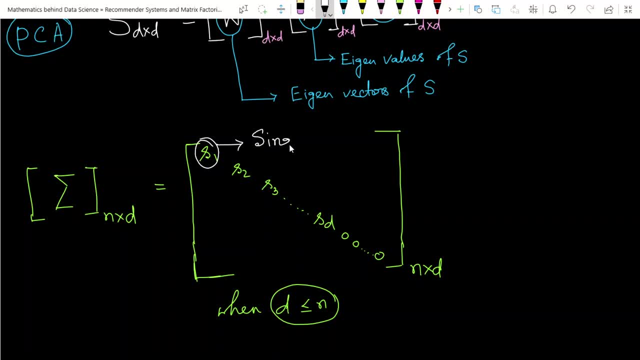 these values are called the singular values of x. these values are called the singular. these values are called the singular. these values are called the singular values. these values are called the singular. these values are called the singular. these values are called the singular values of s, and this is a diagonal matrix. 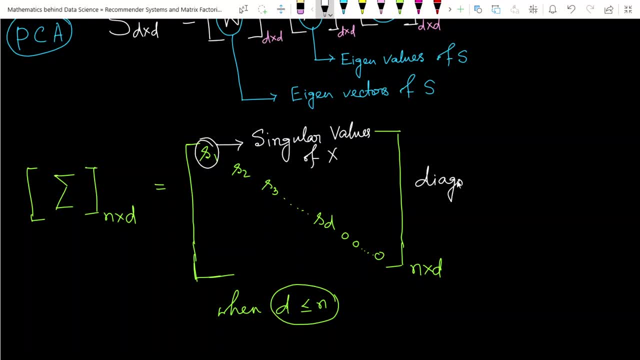 values of s, and this is a diagonal matrix- values of s and this is a diagonal matrix. okay, i think you got the answer now. how okay, i think you got the answer now. how okay, i think you got the answer now. how this, this, this singular singular values are related to: 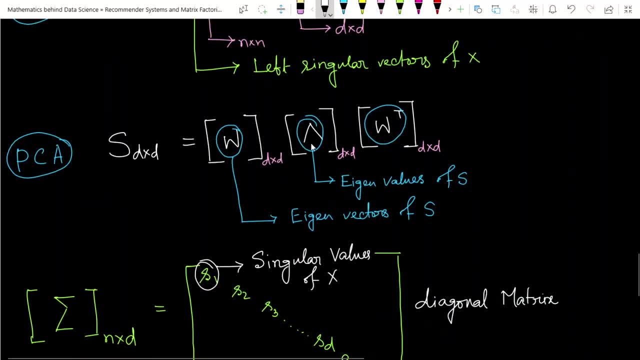 singular singular values are related to singular singular values are related to this. this, this, eigenvalues- this is the main main thing. eigenvalues- this is the main main thing. eigenvalues- this is the main main thing that we have to connect that. we have to connect that. we have to connect how these things are related to this. 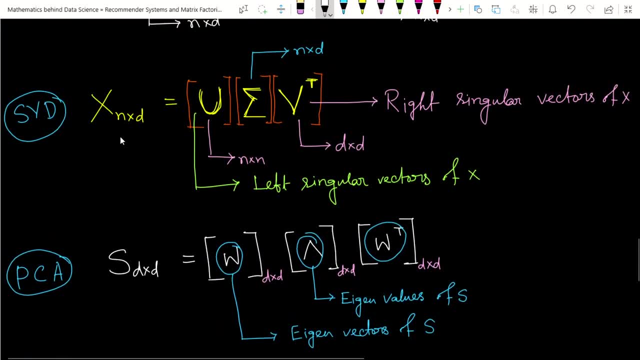 how these things are related to this, how these things are related to this: eigenvalue, eigenvalue, eigenvalue. this is this for the for any data. this is this for the for any data. this is this for the for any data matrix, and this is matrix and this is. 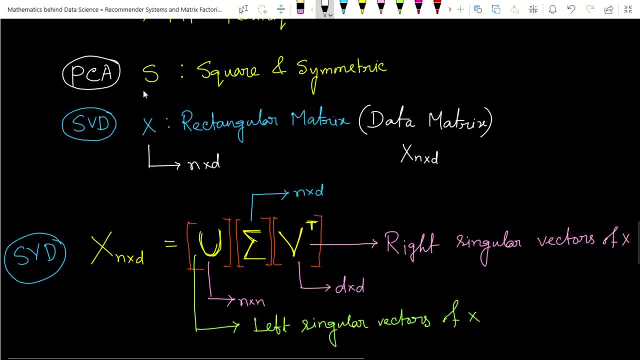 matrix and this is this is matrix and this is this for the. for any data matrix in pca, we use the only matrix and this is this for the. for any data matrix in pca, we use the only matrix and this is this for the. for any data matrix in pca, we use the only covariance matrix in pca, we have. 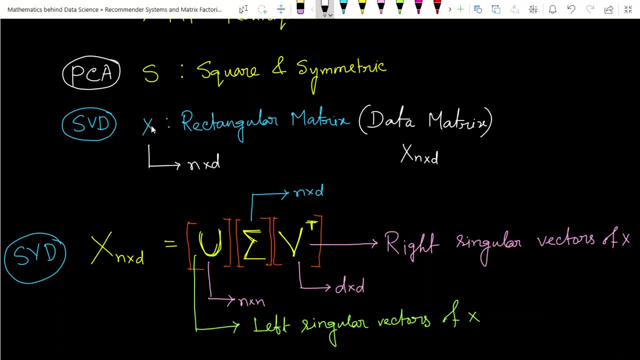 covariance matrix in pca. we have covariance matrix in pca. we have used the covariance matrix, but here we used the covariance matrix, but here we used the covariance matrix. but here we have used, have used, have used any data matrix. now the main thing is any data matrix. now the main thing is: 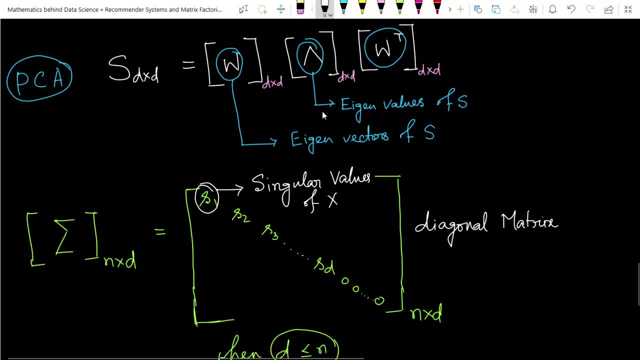 any data matrix. now, the main thing is how to connect this dot. how to connect this dot. how to connect this dot. how this is i is related to the eigen. how this is- i is related to the eigen. how this is i is related to the eigen values of s. 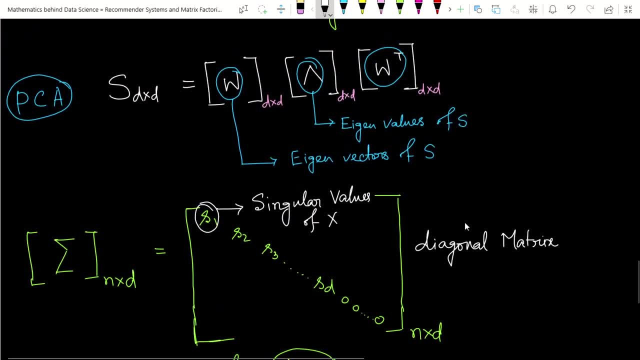 values of s, values of s. that is the main job. so the relations, that is the main job. so the relations, that is the main job. so the relations between these two, between these two, between these two relations now the relations between relations, now, the relations between relations, now the relations between eigenvalues of s. 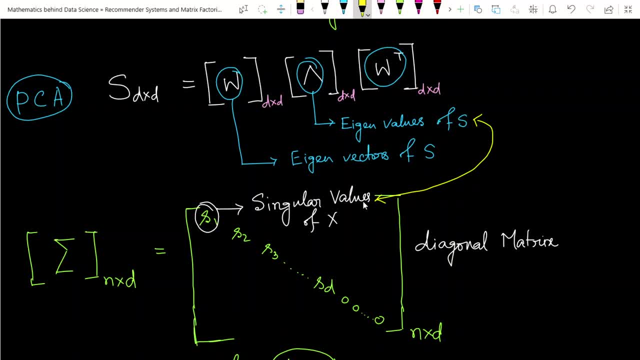 eigenvalues of s. eigenvalues of s and the singular values of and the singular values of and the singular values of x. singular values of x. the relations is x. singular values of x. the relations is x. singular values of x. the relations is the s i square. 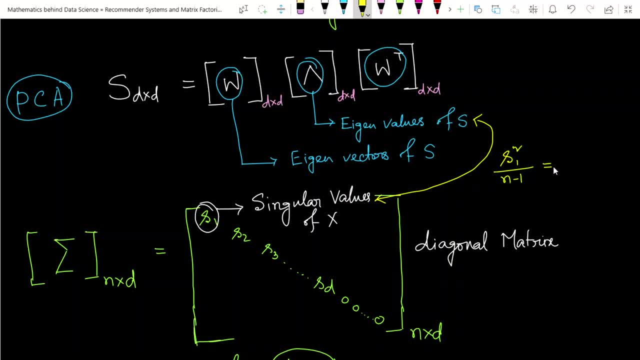 the s i square, the s i square by the n minus 1, by the n minus 1, by the n minus 1 is equals to, is equals to, is equals to lambda i. these are the relations lambda i. these are the relations lambda i. these are the relations between these two values. 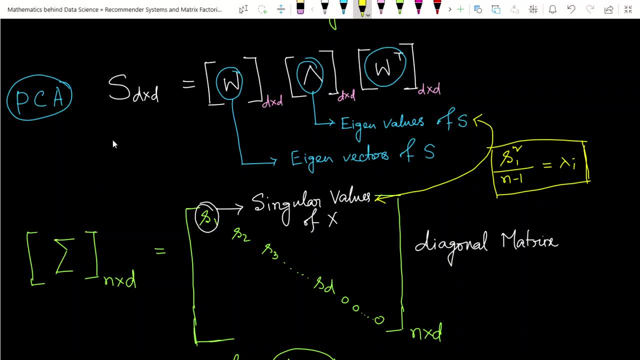 between these two values, between these two values. okay, if we simply take our data sets, okay, if we simply take our data sets, okay, if we simply take our data sets and using simple the matrix factorizations and using simple the matrix factorizations and using simple the matrix factorizations, then we can easily find its. 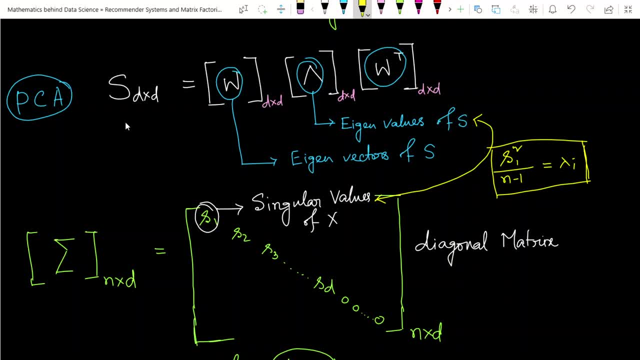 then we can easily find its. then we can easily find its its eigen values, okay, its eigen values, okay, its eigen values, okay, there have no need to calculate it. there have no need to calculate it. there have no need to calculate it. that's the main importance of it. 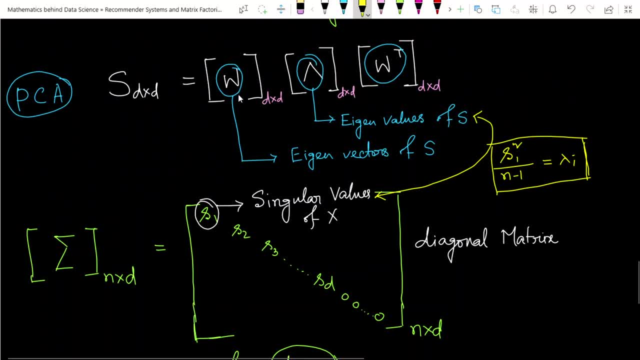 that's the main importance of it. that's the main importance of it. now, let's see what is this significance. now, let's see what is this significance. now, let's see what is this significance of w dot w transpose, let's see it. of w dot w transpose, let's see it. 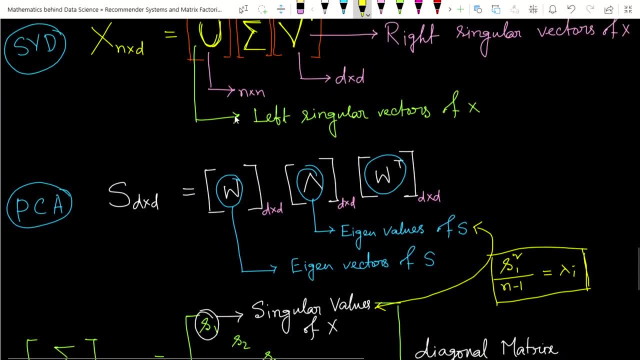 of w dot, w transpose. let's see it so that u i that dot u means here. so that u i that dot u means here. so that u i that dot u means here is in w we got it u and w transpose. we is in w we got it u and w transpose we. 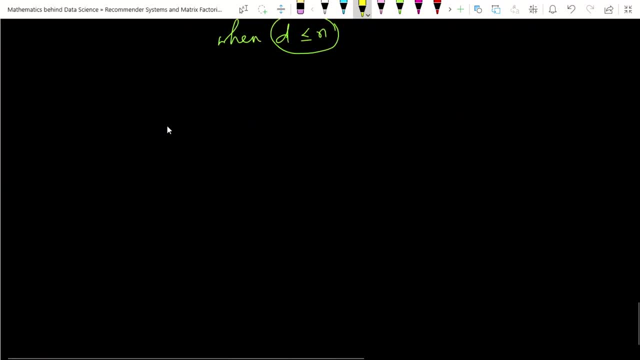 is in: w. we got it u and w transpose. we got it v transpose. so let's see what is got it v transpose. so let's see what is got it v transpose. so let's see what is the importance of u, the importance of u, the importance of u. so the u- we got it. 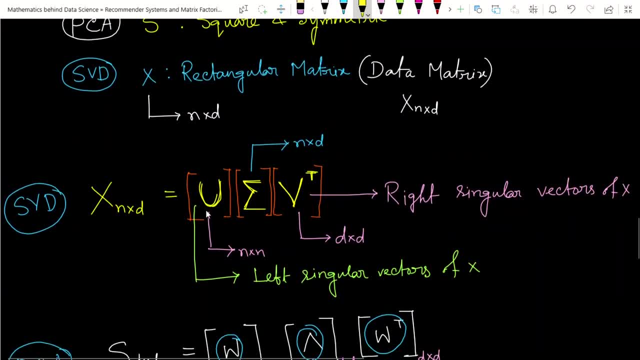 this is the u matrix. what is the? this is the u matrix. what is the? this is the u matrix. what is the dimension of u? dimension of u? dimension of u? and the dimension is n cross n here the. and the dimension is n cross n here the 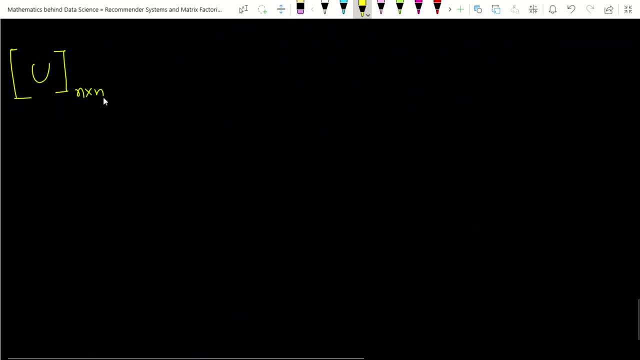 and the dimension is n cross n here. the dimension of is? u is equals to dimension of is u is equals to dimension of is u is equals to n cross n here. this is let the first column of you here. this is let the first column of you. 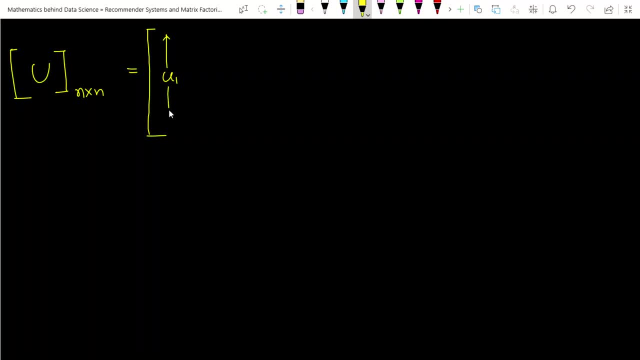 here. this is let the first column of you. this is the u1. this is the first column. this is the u1. this is the first column. this is the u1. this is the first column. right right, right, then it is the first column u2. it's the 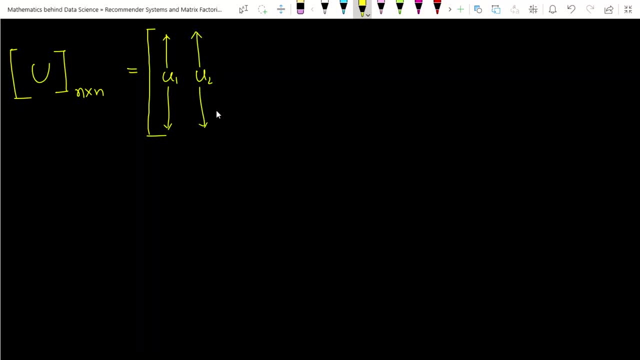 then it is the first column. u2. it's the. then it is the first column. u2. it's the second column. let let u3. it's the third column. like that, since it is n crossing u n. like that, since it is n crossing u n. 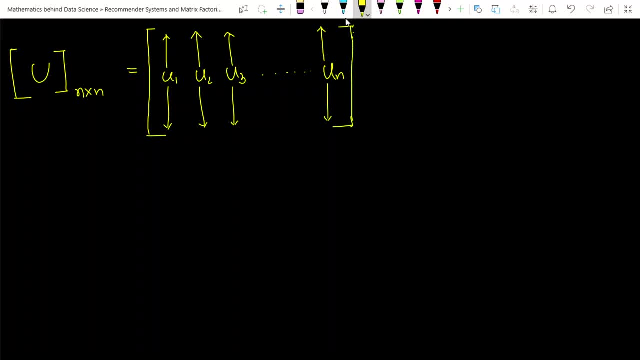 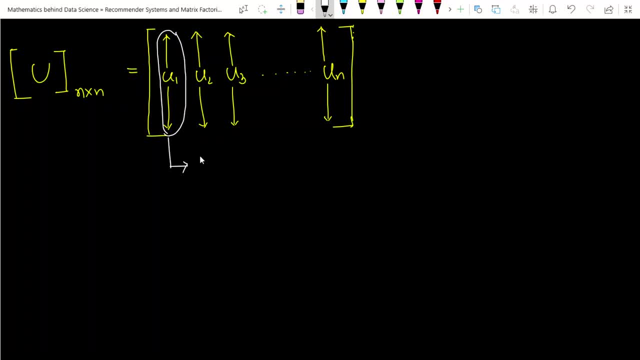 the dimension. here it will be. here. the dimension is dimension is dimension is. its dimensional is: it's a single column. n its dimensional is: it's a single column. n its dimensional is: it's a single column n rows. the dimension is n cross one rows. the dimension is n cross one. 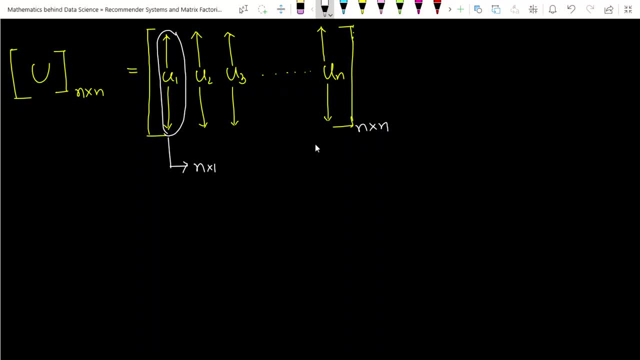 rows. the dimension is n cross one. its dimension is n crossing. its dimension is n crossing. its dimension is n crossing. okay, now, this height, this height, this okay, now, this height, this height, this, okay, now, this height, this height. this column is called the. this column of u is: 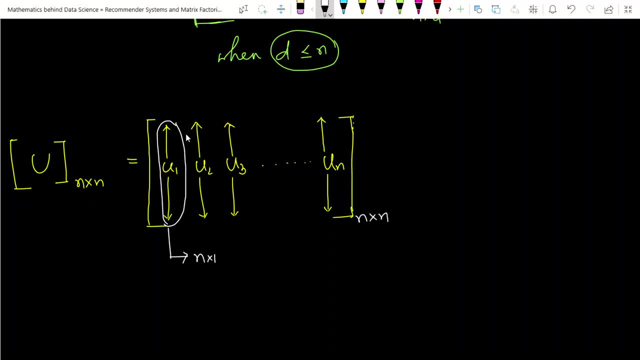 column is called the. this column of u is column is called the. this column of u is called the called the. called the eigenvector of. eigenvector of. eigenvector of of x- comma x. transpose x- x into x. of x- comma x. transpose x- x into x. 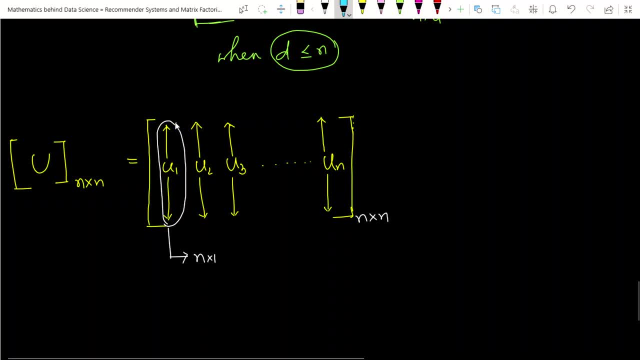 of x comma x. transpose x- x into x. transpose, transpose, transpose. okay, these things are actually called okay. these things are actually called okay. these things are actually called the eigenvectors of x comma x- transpose eigenvectors of it. x comma x- transpose eigenvectors of it. 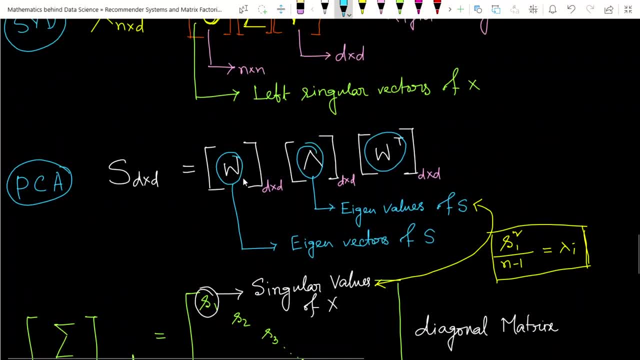 x, comma x transpose eigenvectors of it. so okay, so okay, so okay. but here it is like what, but here it is like what, but here it is like what it is called, it is called, it is called in pca, where you see it, the eigenvectors. 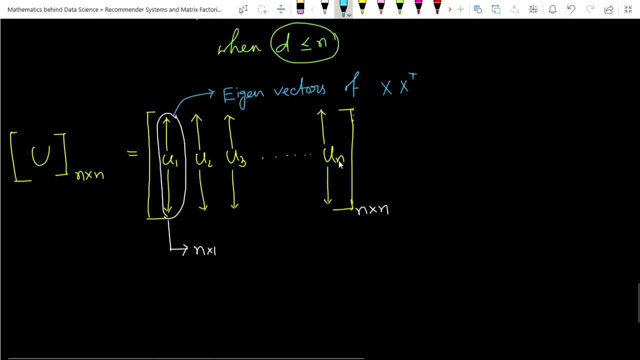 in pca, where you see it, the eigenvectors in pca, where you see it, the eigenvectors of simple s, of simple s, of simple s, but here it, instead of using s, it's the, but here it, instead of using s, it's the, but here it, instead of using s, it's the eigenvector of x into x transpose. so 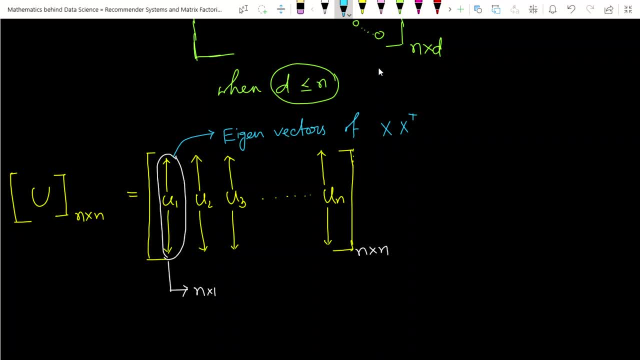 eigenvector of x into x transpose. so, eigenvector of x into x transpose. so let's see it's dimensional mass or not? let's see it's dimensional mass or not? let's see it's dimensional mass or not? so what is the dimension of x? 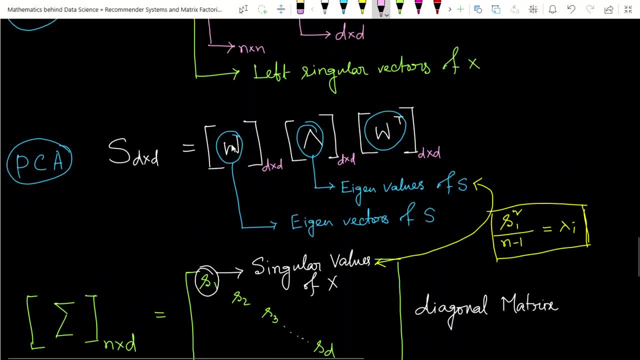 so what is the dimension of x? so what is the dimension of x? remember. the dimension of x is what remember. the dimension of x is what remember. the dimension of x is what. let's see. dimension of x is n cross d. let's see: dimension of x is n cross d. 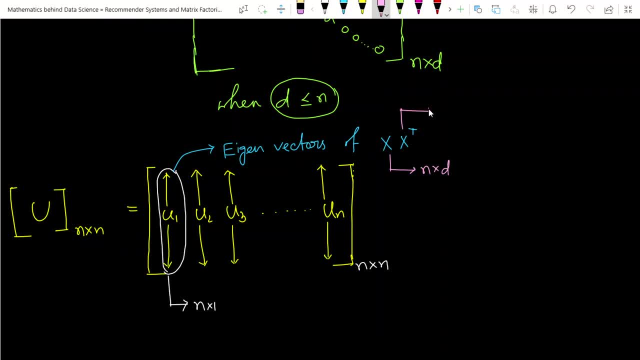 let's see: dimension of x is n cross d, its dimensional is n cross d. its dimensional is n cross d. its dimensional is n cross d. and x transpose its dimensional will be: and x transpose its dimensional will be: and x transpose its dimensional will be d cross n. 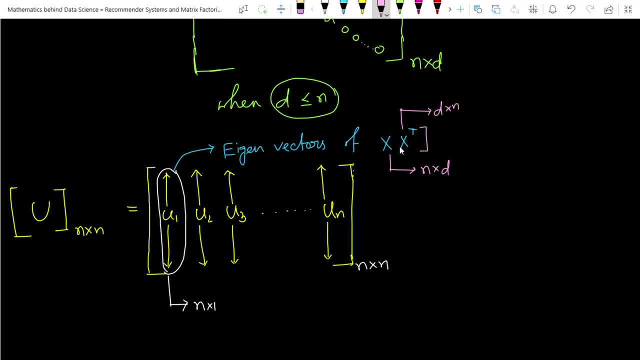 d cross n, d cross n. if you see, if we just start doing the job, if you see, if we just start doing the job, if you see, if we just start doing the job multiplication, the job multiplication, the job multiplication, the job, then its dimensional will be n cross n. 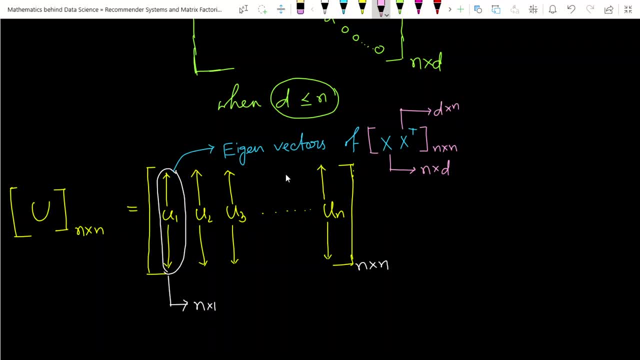 then its dimensional will be n cross n. then its dimensional will be n cross n. okay, that's the both that the same. okay, that's the both that the same. okay, that's the both that the same. dimension, dimension, dimension. okay, it's possible to find the eigen. 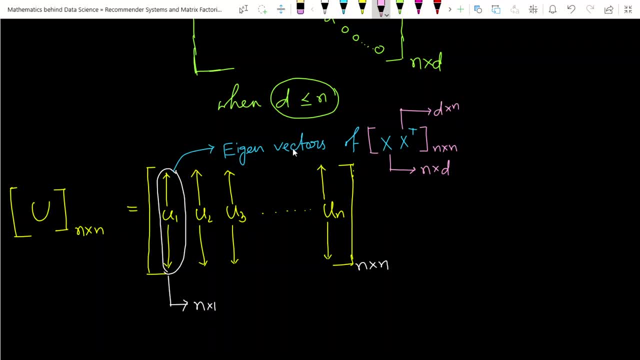 okay, it's possible to find the eigen. okay, it's possible to find the eigen vector. this, h, ui, these h column vectors, vector this, h, ui, these h column vectors, vector this, h, ui, these h column vectors are called the eigen vectors, are called the eigen vectors, are called the eigen vectors of our this x into x transpose, that's. 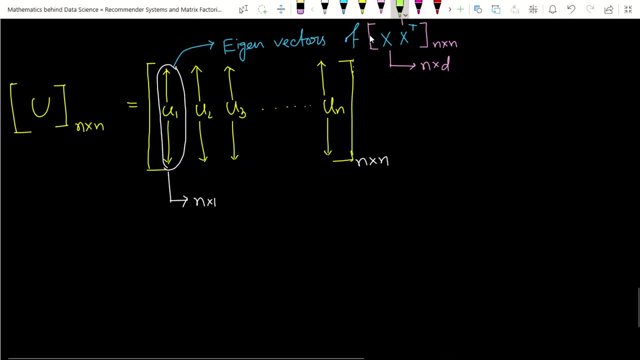 of our this x into x transpose, that's of our this x into x transpose. that's the important importance now. let's see the important importance now. let's see the important importance now. let's see. the same things also applicable for v. the same things also applicable for v. 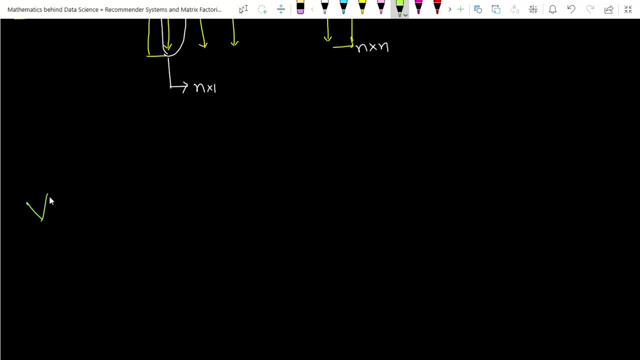 the same things also applicable for v, v, v, v, so v will be, so v will be, so v will be v. suppose let's, instead of using the v v, suppose let's, instead of using the v v, suppose let's, instead of using the v v, transpose here i have used the b symbol. 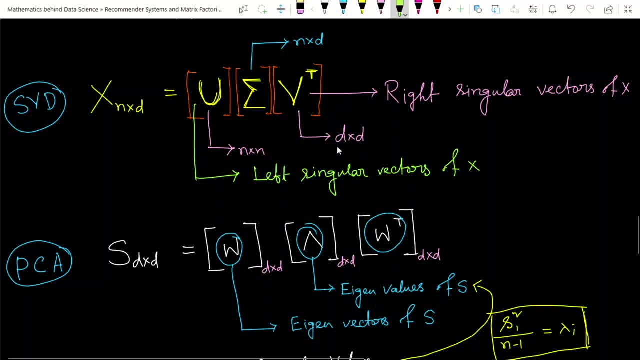 v transpose- here i have used the b symbol. v transpose- here i have used the b symbol. better for us v is how much dimensional. better for us v is how much dimensional. better for us v is how much dimensional v is. d cross d dimension, so it's v. 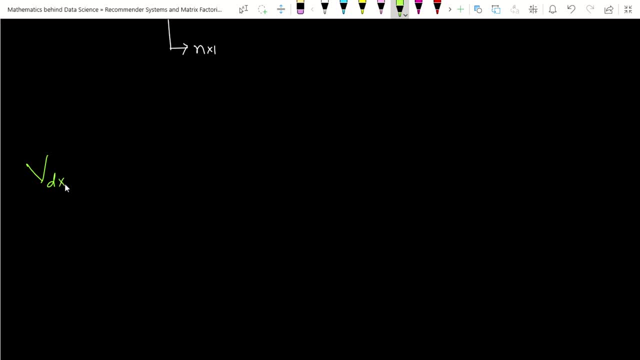 v is d cross d dimension, so it's v. v is d cross d dimension, so it's v transpose, v transpose is d cross d transpose. v transpose is d cross d transpose. v transpose is d cross d dimension. so v will be like same dimension, so v will be like same. 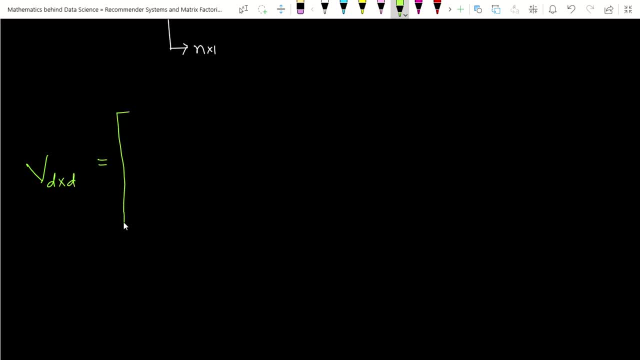 dimension. so v will be like same d cross d diamond. let's, it is the v1. it's v2 column. v3. let's, it is the v1. it's v2 column. v3- let's, it is the v1. it's v2 column. v3 column. 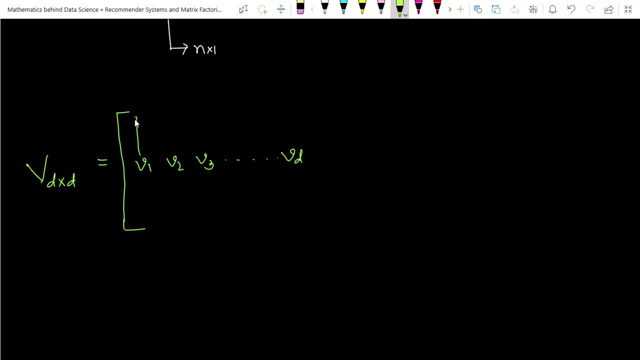 column column like that to vd. column like that to vd column. like this kind of matrix, we got like this kind of matrix, we got like this kind of matrix, we got. okay, this is the d cross d and the dimension of the h vector. it's and the dimension of the h vector: it's. 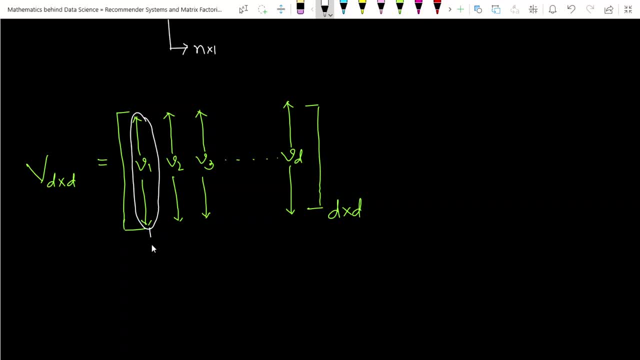 and the dimension of the h vector. it's the column vector of v, the column vector of v, the column vector of v. it's the column vector and the dimension. it's the column vector and the dimension. it's the column vector and the dimension. its dimension will be. 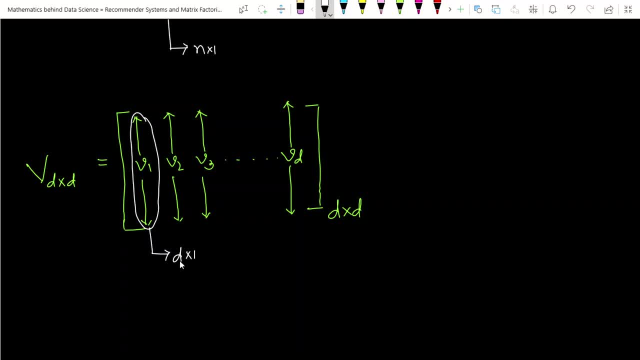 its dimension will be. its dimension will be its d dimension into one, its d dimension into one, its d dimension into one d row and single d row and single d row and single column. and these the importance of it column, and these the importance of it column, and these the importance of it. it's the eigenvector of. 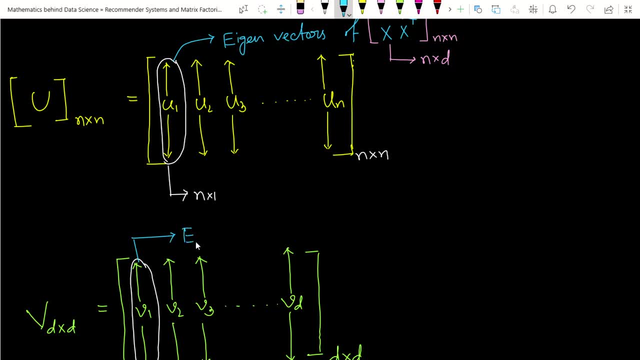 it's the eigenvector of it's the eigenvector of importance of this h column vector, is importance of this h column vector, is importance of this h column vector is the it is this also. it's called a. it's also called a eigenvectors or. 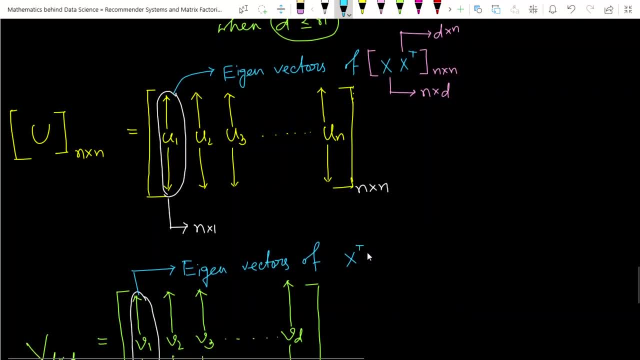 it's also called a eigenvectors. or it's also called a eigenvectors, or, but in same opposite: multiplication x, but in same opposite multiplication x, but in same opposite: multiplication x, transpose, x, transpose, x transpose, x, x, transpose. let's see what will be its. 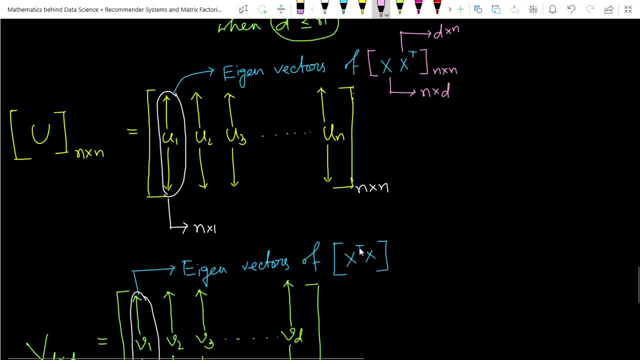 x transpose. let's see what will be its x transpose. let's see what will be its dimension, dimension, dimension, so the dimension of x transpose. so the dimension of x transpose. so the dimension of x transpose. dimension of the x transpose is what? dimension of x is what. 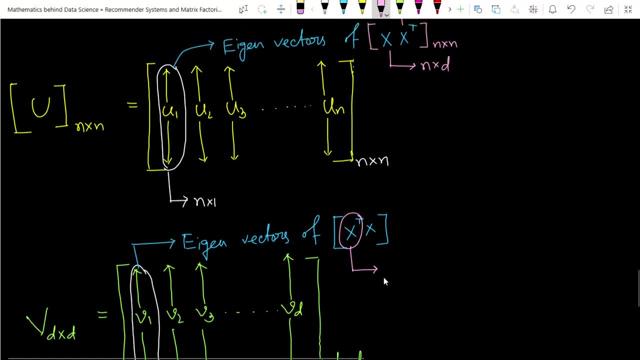 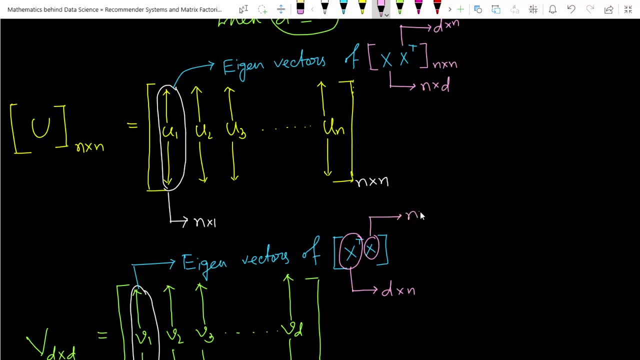 dimension of x is what dimension of x? transpose it will be d. dimension of x: transpose it will be d dimension of x. transpose it will be d cross n and dimension of x is and dimension of x is. and dimension of x is n cross d. if we're doing the 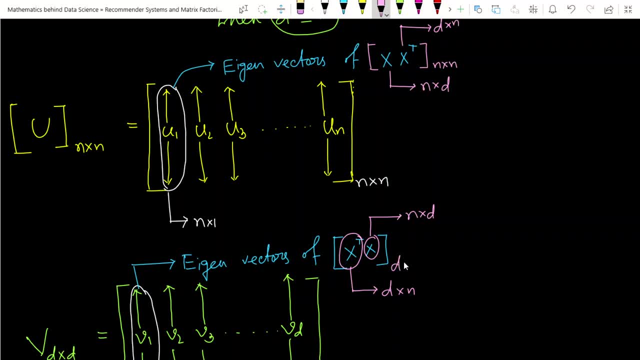 n cross d, if we're doing the n cross d, if we're doing the multiplications between them, then we got multiplications between them. then we got multiplications between them. then we got d cross d matrix, d cross d matrix, d cross d matrix, then we got d cross d matrix. example this: 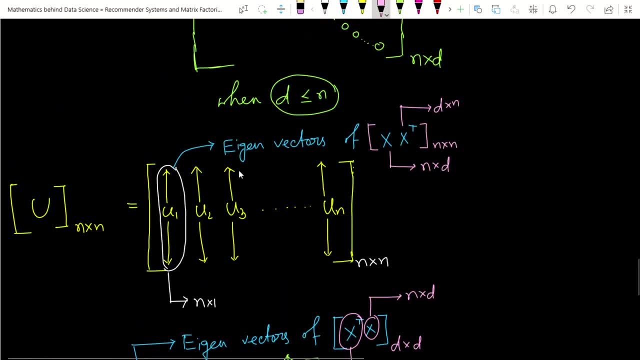 then we got d cross d matrix example: this: then we got d cross d matrix example. this is the eigenvectors of x. transpose x is the eigenvectors of x. transpose x is the eigenvectors of x- transpose x. and these are the eigenvectors of x- x. 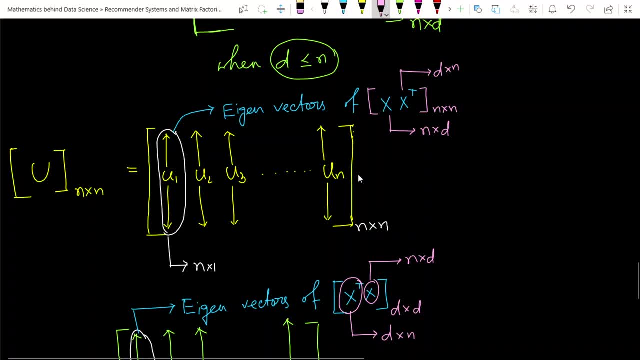 and these are the eigenvectors of x, x, and these are the eigenvectors of x, x. transpose x into x. transpose- okay, that's. transpose x into x. transpose- okay, that's transpose x into x. transpose- okay. that's the importance of the singular value, the importance of the singular value. 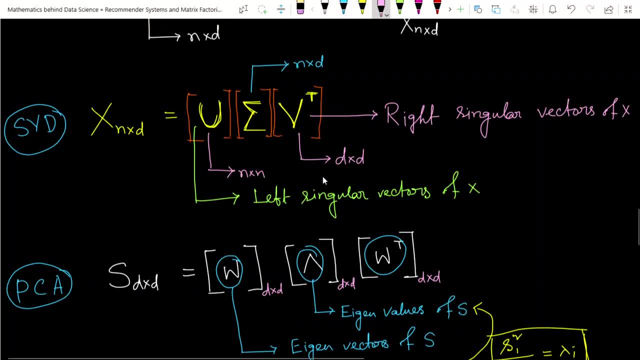 the importance of the singular value. decompositions: both are the same things. decompositions: both are the same things. decompositions- both are the same things. actually, at the end of the day board, actually at the end of the day board, actually at the end of the day board- will do the same thing. 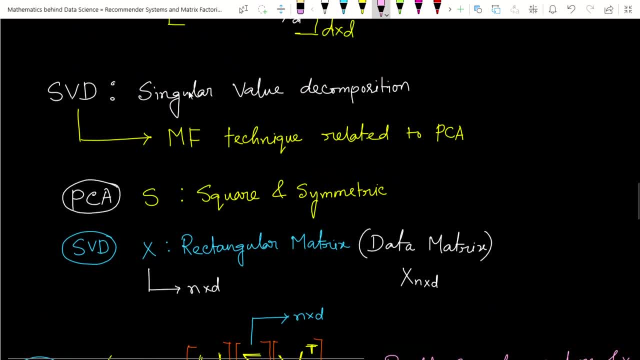 will do the same thing, will do the same thing in pcf first. we have to calculate the in pcf first. we have to calculate the in pcf first. we have to calculate the uh covariance matrix, but in singular uh covariance matrix, but in singular uh covariance matrix, but in singular value decompositions. if we apply it, we 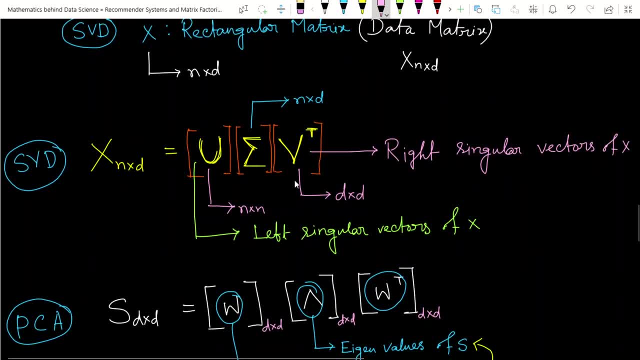 value decompositions if we apply it. we value decompositions if we apply it. we can direct you can. you can easily can direct you can. you can easily can direct you can. you can easily direct find the direct, find the direct, find the eigenvectors and eigenvalue. there are no. 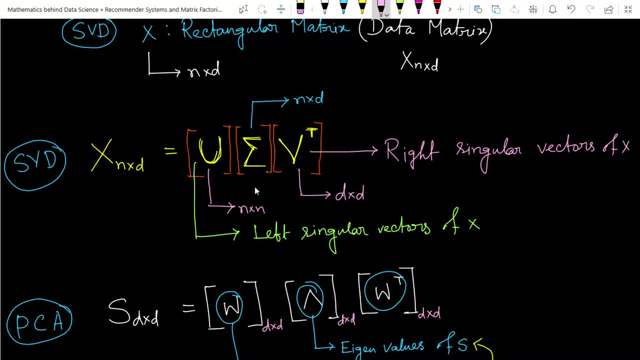 eigenvectors and eigenvalue. there are no eigenvectors and eigenvalue. there are no need to find, the need to find, the need to find the, and that is in the covariance matrix and that is in the covariance matrix and that is in the covariance matrix. okay, 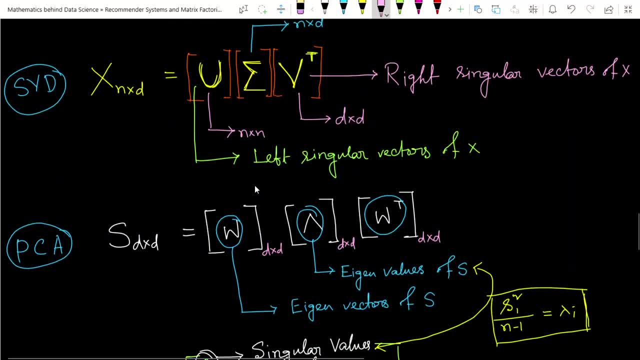 okay, okay, that is the main important thing here. that is the main important thing here. that is the main important thing here. i think you got the answer. i think you got the answer. i think you got the answer. so, if you just summarize this thing, if so, if you just summarize this thing, if, 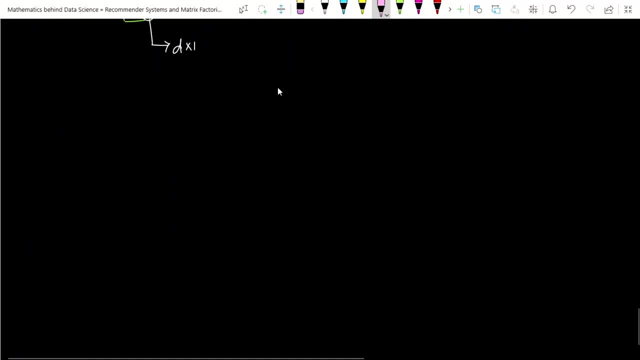 so if you just summarize this thing, if you just summarized, you just summarized, you just summarized this thing, that we have got so in this thing, that we have got so in this thing, that we have got so in first in pca, first in pca, first in pca, if you just summarize this thing, that 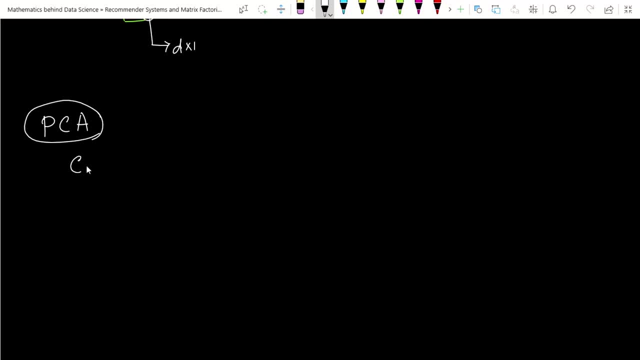 if you just summarize this thing, that, if you just summarize this thing that we have learned in pca what we have. we have learned in pca what we have. we have learned in pca what we have seen in pcf first. we have seen in pcf first we have. 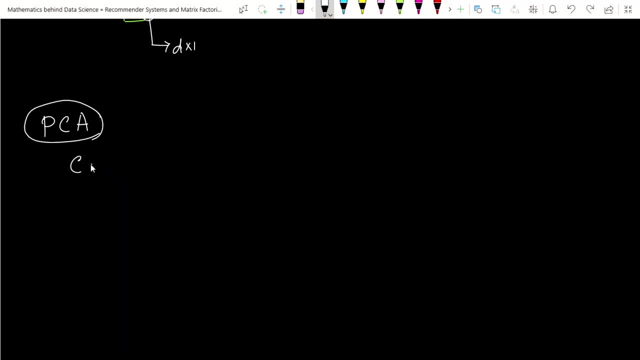 seen in pcf. first we have on calculate, calculate the covariance on calculate, calculate the covariance on calculate, calculate the covariance matrix, matrix matrix. first we calculate the covariance matrix. first we calculate the covariance matrix. first we calculate the covariance matrix of the, of the, of the data matrix x we got it is: 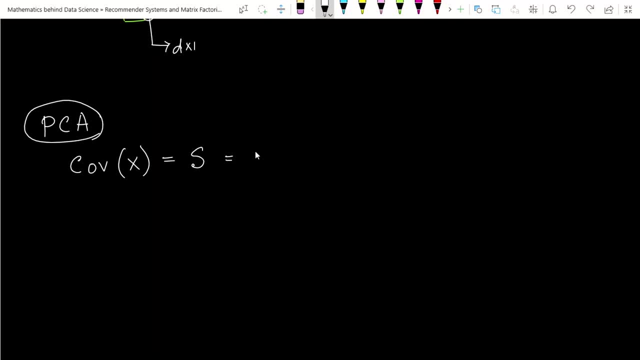 data matrix x we got. it is data matrix x we got. it is s. and by simple using s and it's s, and by simple using s and it's s, and by simple using s and it's after after matrix factorizations we, after after matrix factorizations: we. 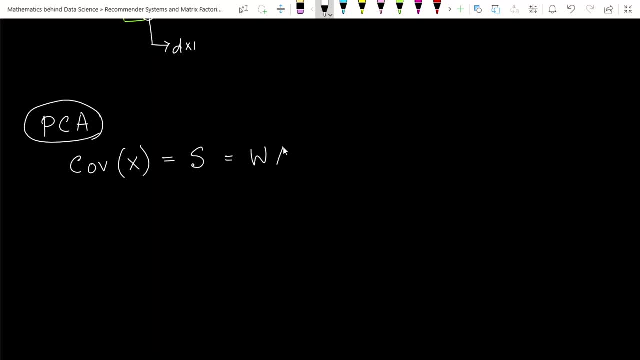 after, after matrix factorizations. we got this easy, like got this easy, like got this easy. like w capital w capital w capital gamma w transpose gamma w transpose gamma, w transpose okay that matrix and the importance of okay that matrix and the importance of okay that matrix and the importance of this w is. 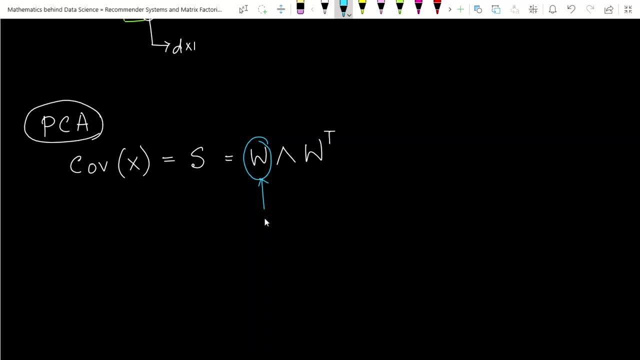 this w is. this w is the w's are give us. gives us the eigen the w's are give us. gives us the eigen the w's are give us. gives us the eigen vectors. this w gives us the eigen vectors. this w gives us the eigen vectors. 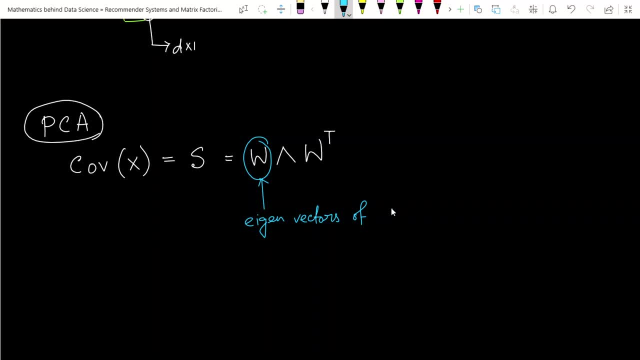 this w gives us the eigen vectors of the covariance matrix. is of the covariance matrix, is of the covariance matrix, is okay, okay, okay. and this and this and this lambda, this lambda are gives us the lambda. this lambda are gives us the lambda, this lambda are gives us the eigen values. this lambda gives us the. 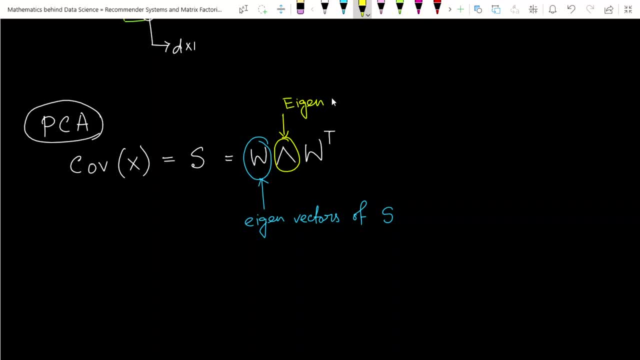 eigen values. this lambda gives us the eigen values. this lambda gives us the eigen values. eigen values of the covariance matrix is eigen values of the covariance matrix. is eigen values of the covariance matrix is okay, that is the importance of it. okay, that is the importance of it. 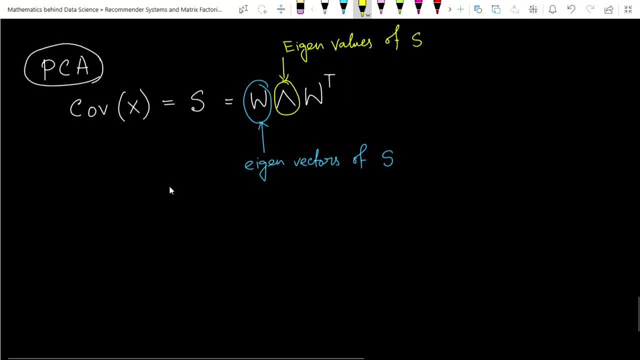 okay, that is the importance of it, eigen values of eigen values of it, eigen values of it, eigen values of it. that's we have seen in pca, but that's we have seen in pca, but that's we have seen in pca. but in, if you use this thing, same things. 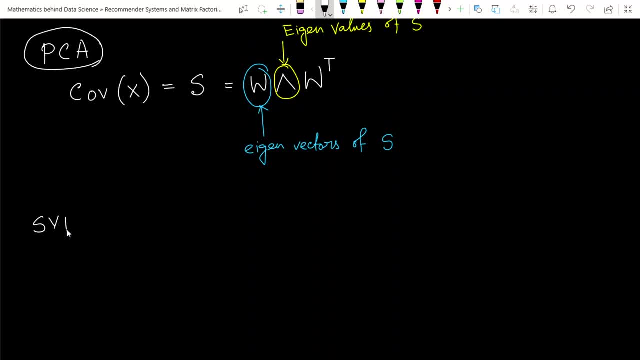 in. if you use this thing, same things in. if you use this thing, same things also. if we use in singular value to also, if we use in singular value to also. if we use in singular value to decomposition technique, decomposition technique, decomposition technique, then instead of use the finding, the 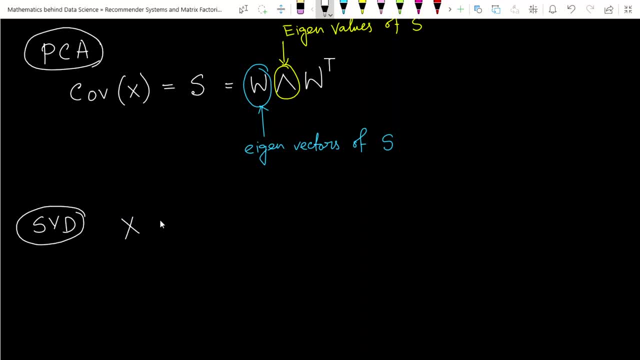 then, instead of use the finding the, then, instead of use the finding, the covariance, we have direct use this in x covariance. we have direct use this in x covariance. we have direct use this in x. to this into the matrix factorization, to this into the matrix factorization. 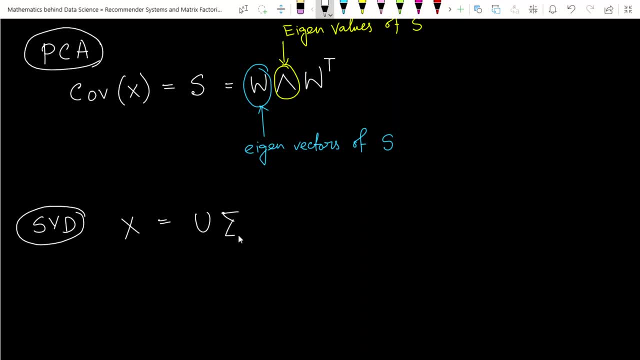 to this into the matrix factorization technique, technique, technique. but u sigma v transpose, but u sigma v transpose, but u sigma v transpose. so the, so the, so the, the sigma here. the sigma here gives us the sigma here. the sigma here gives us the sigma here, the sigma here gives us the singular values. these gives us the. 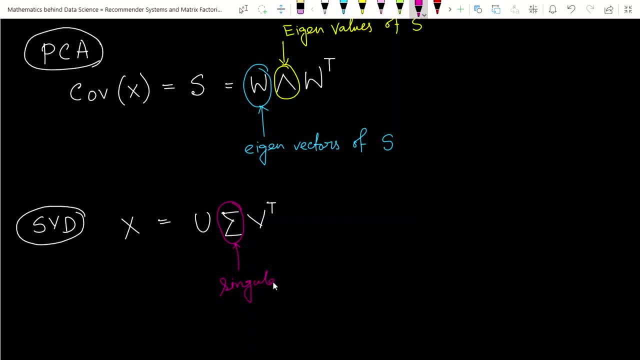 singular values. these gives us the singular values, these gives us the singular values, since si this gives us the singular, since si this gives us the singular, since si this gives us the singular values is i and the relations between values is i and the relations between values is i and the relations between these eigen values and the singular. 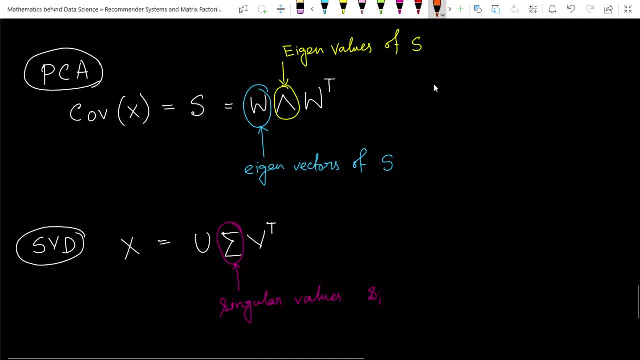 these eigen values and the singular, these eigen values and the singular values and relations between it values and relations between it values and relations between it is like that is like. that is like that: the relations between is is i, the relations between is is i, the relations between is is i is i square by. 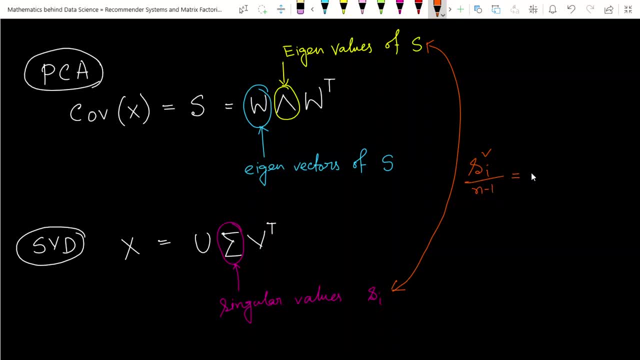 is i square by? is i square by? n minus one? n minus one? n minus one simply equals to lambda i simply equals to lambda. i simply equals to lambda i. that is the relations we got we have. that is the relations we got we have. that is the relations we got we have find. 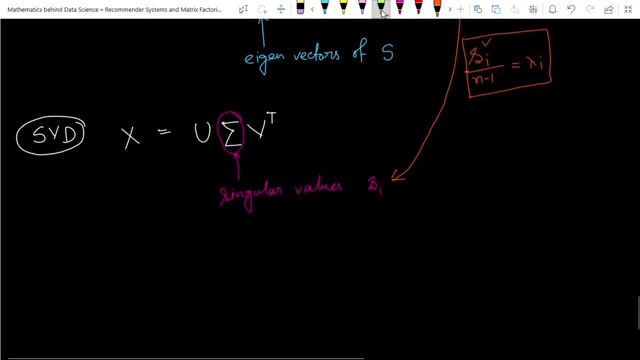 find, find and the ui here ui and the ui here ui and the ui here ui gives us the this u and v gives us the this u and v gives us the this u and v, this u, this u, this u or. it gives us the sample, the eigen. 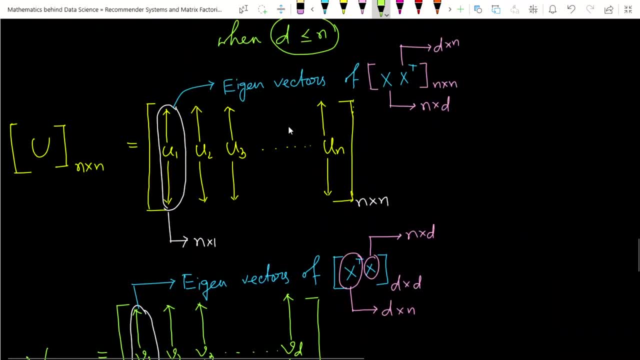 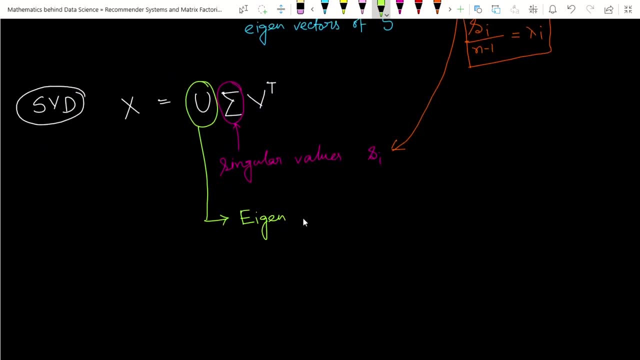 or it gives us the sample, the eigen, or it gives us the sample, the eigen vectors. these are: gives us the eigen vectors. these are: gives us the eigen vectors. these are: gives us the eigen vectors of vectors, of vectors of x into x transpose. this keeps as the. 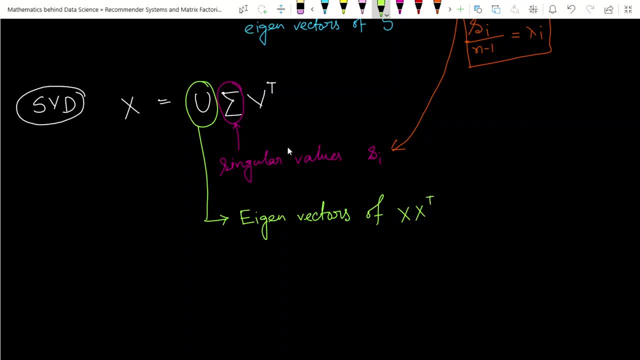 i against vectors of x and x transpose. i against vectors of x and x transpose. i against vectors of x and x transpose. and this v- transpose gives us these extras, gives us the eigen vectors. these extras gives us the eigen vectors. these extras gives us the eigen vectors of: 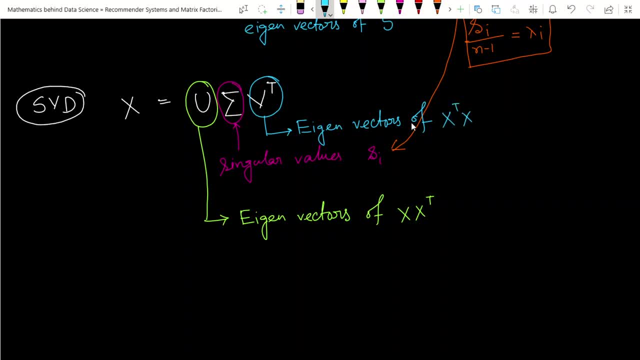 just just these extras gives us the eigen vectors of x transpose x, of x transpose x, of x transpose x. but that is the job that we have seen here. but that is the job that we have seen here. but that is the job that we have seen here. that is the thing i'm doing. both are 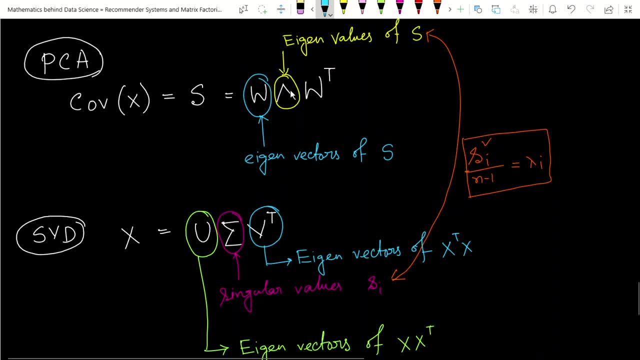 that is the thing i'm doing. both are. that is the thing i'm doing. both are there at the end of the board. are the there at the end of the board? are the there at the end of the board? are the same border? that both are the? 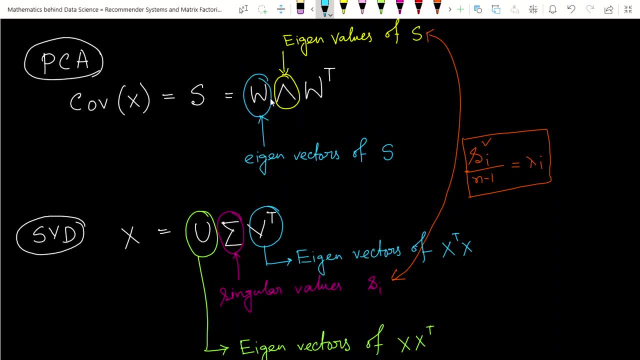 same border, that both are the same border, that both are the applications of matrix factorizations, applications of matrix factorizations, applications of matrix factorizations, but in different point of view, but in different point of view, but in different point of view. so i think the s? vd techniques are more 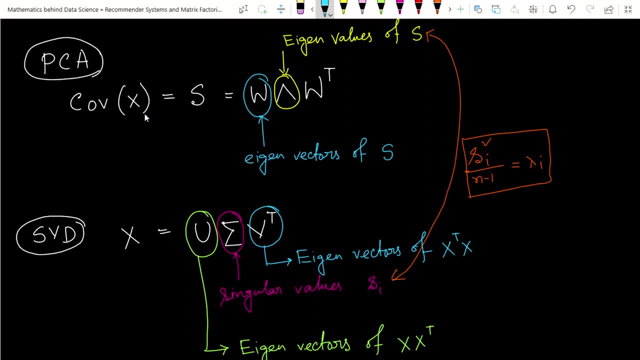 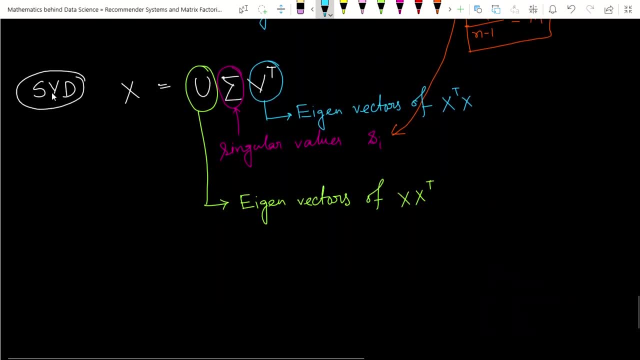 so i think the s? vd techniques are more so, i think the s? vd techniques are more easy, easy, easy, okay, so that we have seen here, we have okay, so that we have seen here, we have okay, so that we have seen here, we have connect the dots and the end of this. 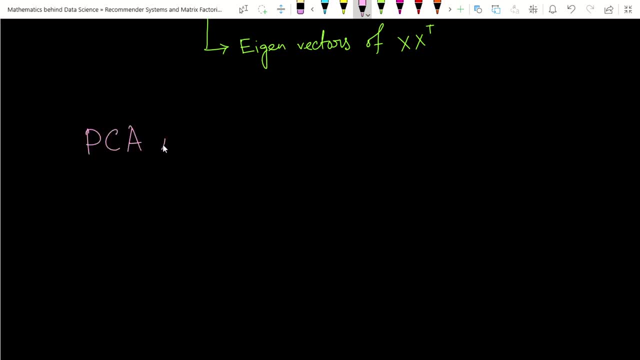 connect the dots and the end of this. connect the dots and the end of this lecture. we lecture, we lecture, we connect the dots. this pca will connect. connect the dots. this pca will connect. connect the dots. this pca will connect the dots, the the dots, the singular value, decomposition. 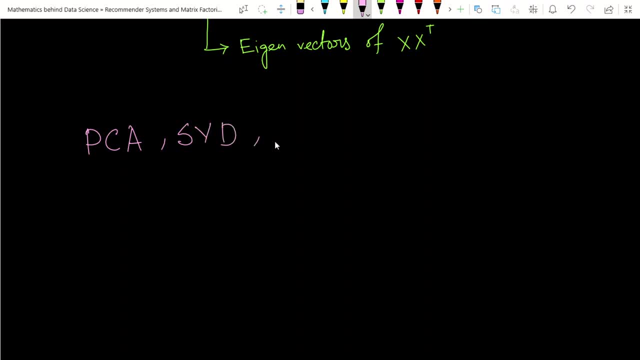 the dots, the singular value, decomposition, the dots, the singular value, decomposition, technique, technique, technique and and connect these two things into and. and connect these two things into and. and connect these two things into the matrix factorization, the matrix factorization, the matrix factorization, the. how much important it in matrix. 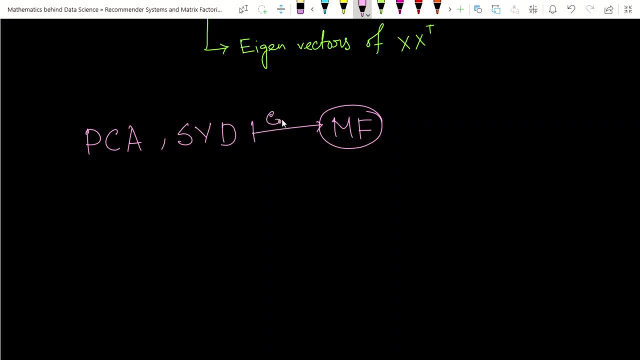 the, how much important it in matrix, the, how much important it in matrix, factorization. so we will factorization, so we will factorization, so we will see the connect it. we will connect it so in future video in. we will connect it so in future video in. 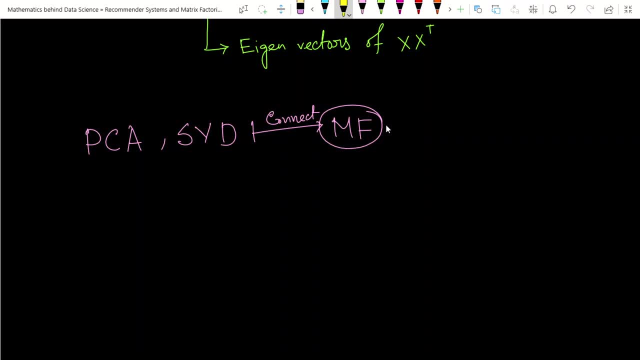 we will connect it. so in future video, in next future video, we will next future video, we will next future video, we will. you will see how to connect this matrix. you will see how to connect this matrix. you will see how to connect this matrix. factorization technique. 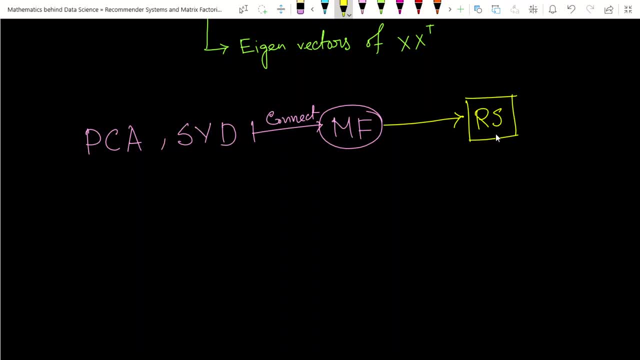 factorization technique, factorization technique with the recommenders recommendation, with the recommenders recommendation, with the recommenders recommendation, system, system, system, how to connect these things? so i think how to connect these things, so i think how to connect these things. so i think matrix factorization is how much. 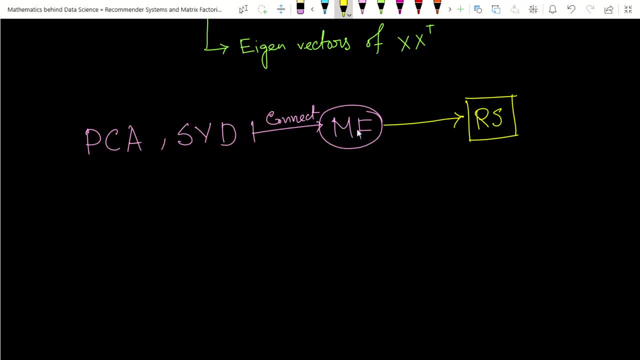 matrix factorization is, how much matrix factorization is how much important. so when important, so when important, so when we also you have seen so in clustering, we also you have seen so in clustering, we also you have seen so in clustering techniques also, we can connect this. 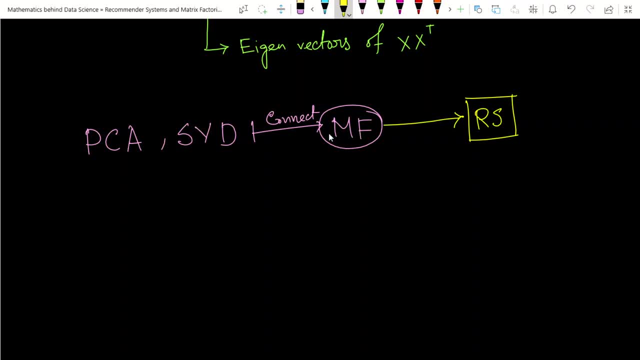 techniques also. we can connect this techniques also. we can connect this matrix factorization to the clustering matrix factorization to the clustering matrix, factorization to the clustering technique as well. technique as well, technique as well. okay, we'll see these things in the next. okay, we'll see these things in the next. okay, we'll see these things in the next in. in the next few videos we will see in. in. in the next few videos we will see in in in the next few videos we will see in this chapter, we will see how this, this chapter, we will see how this. 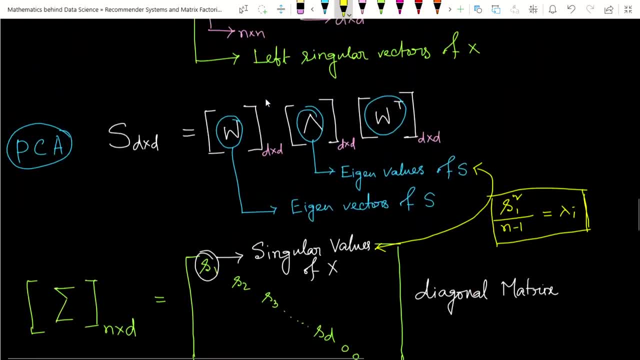 this chapter we will see how this matrix factories and techniques are matrix factories and techniques are matrix factories and techniques are useful in the machine learning. okay, i useful in the machine learning. okay, i useful in the machine learning. okay, i think from this, think from this, think from this discussions, you got the idea how the 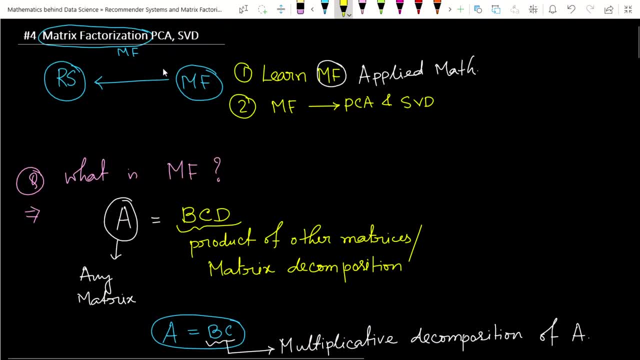 discussions. you got the idea how the discussions. you got the idea how the principal component analysis are actually principal component analysis are actually principal component analysis are actually you work how the matrix factorization you work, how the matrix factorization you work, how the matrix factorization techniques are actually work behind the 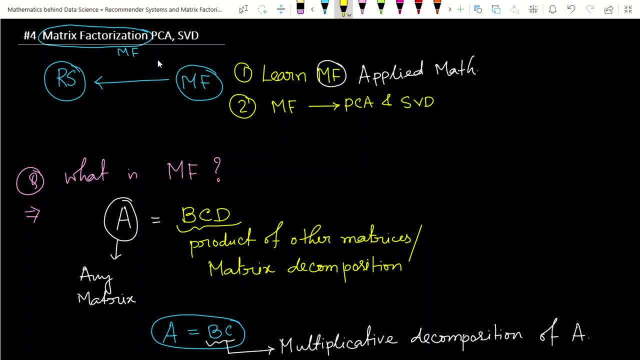 techniques are actually work behind. the techniques are actually work behind the principal component analysis, principal component analysis. principal component analysis: okay, and in next here, the next future: okay, and in next here, the next future, okay, and in next here, the next future video. we will see how this also, how this.